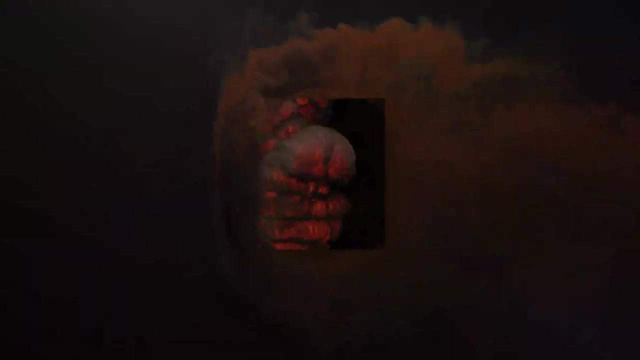 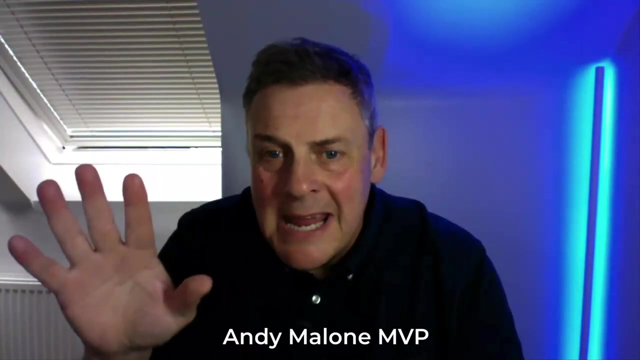 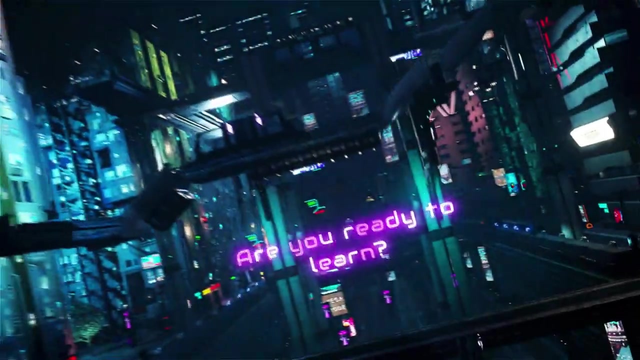 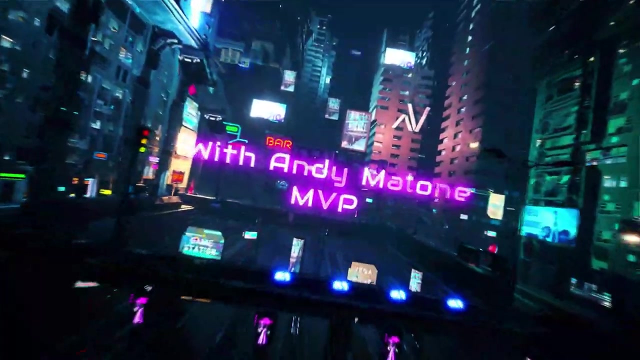 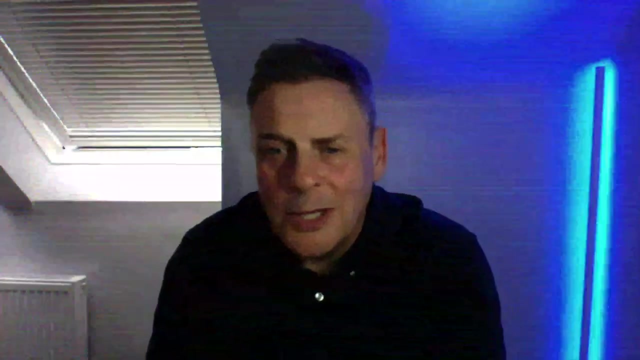 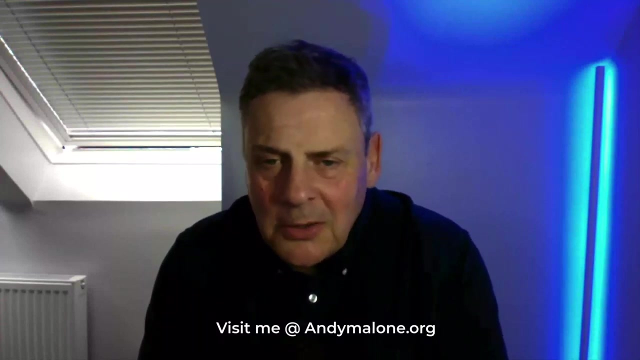 This time around, it's the turn of cryptography made simple- And I do mean simple. So are you ready to learn? Let's take a look. Hi everyone, welcome back to the channel Andy Malone, Microsoft MVP and Microsoft Certified Trainer. This time around, I've got something a little bit different for you. 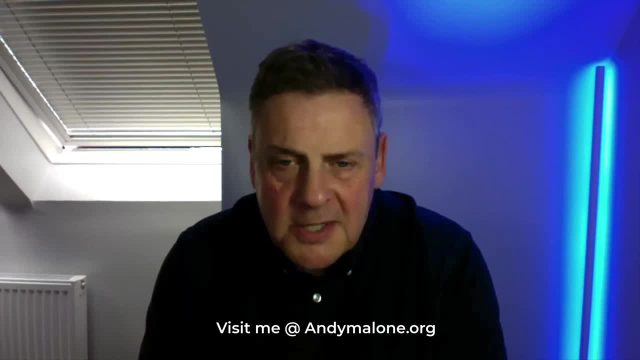 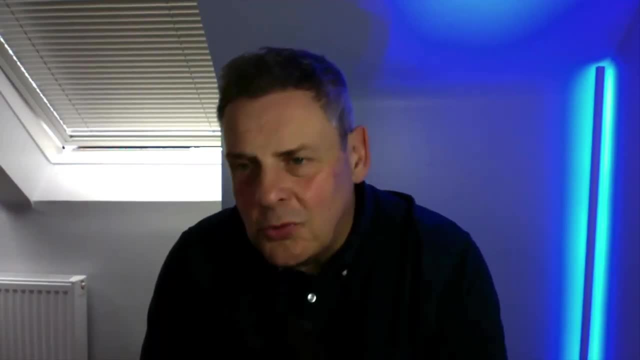 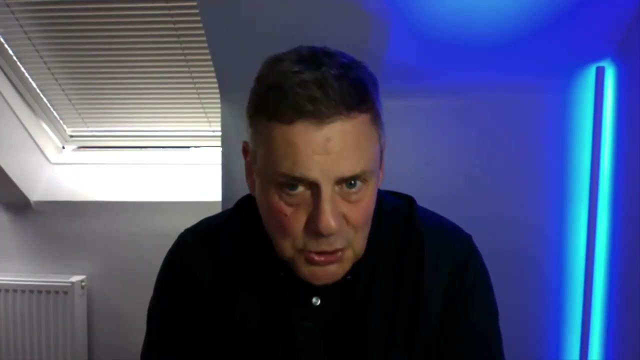 I'm going to take a trip into cryptography and we're going to discuss exactly what it is, how it works, its history and its development. And, of course, we can't talk about this in just one lesson. So, for the first time, I'm actually going to break this down into three separate sessions, So this being part one. 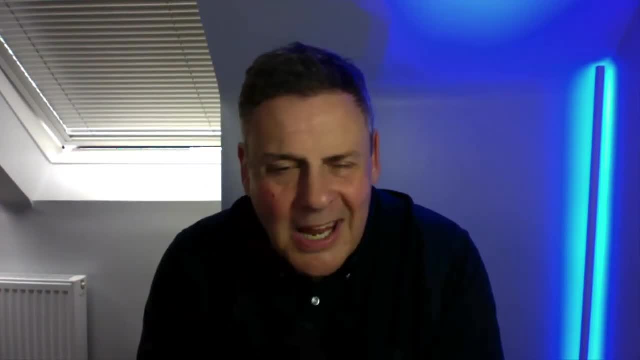 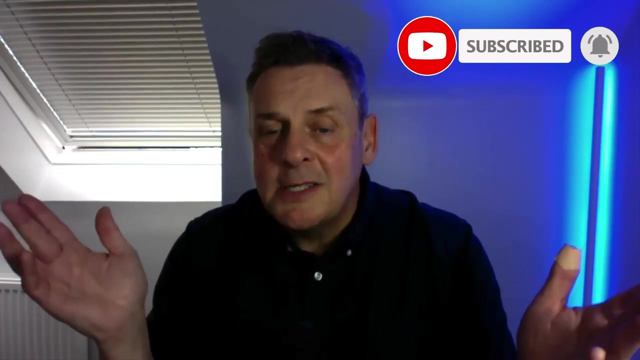 Now, of course, I welcome your feedback. So if you've got any questions at all, then go ahead and pop them down below and I will get to them. So don't worry. As always, if you like what you see, go ahead, hit that subscribe button, ring that bell and you won't miss the future postings. So are you ready to learn? Let's take a look. 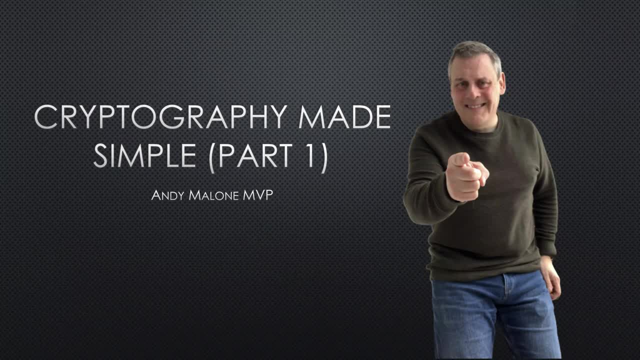 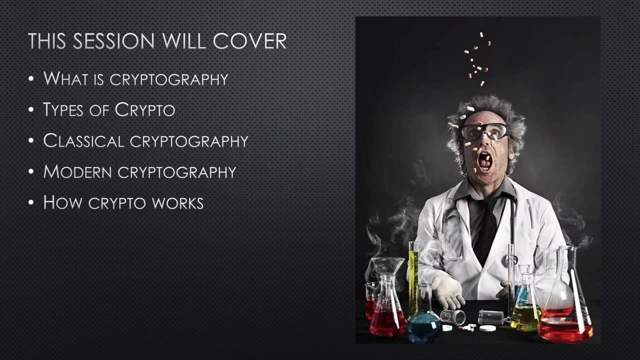 So this is part one of cryptography made simple. So in this session, we're going to talk about exactly what cryptography is. We'll talk about the types of cryptography that we use. We're going to specifically focus on classical cryptography and also modern cryptography and as, of course, also how it works. 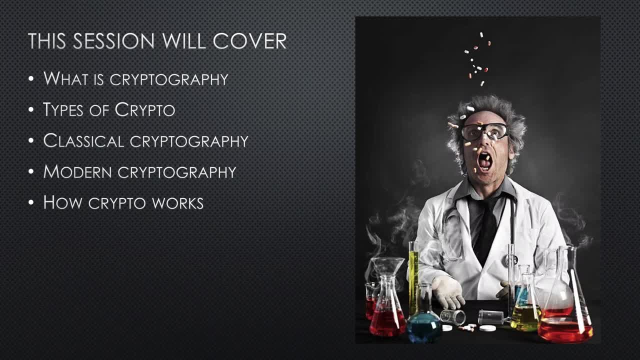 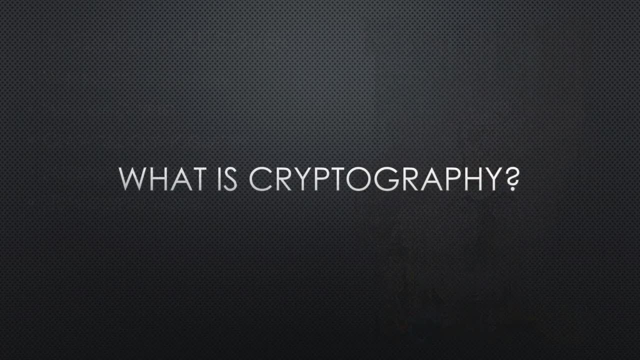 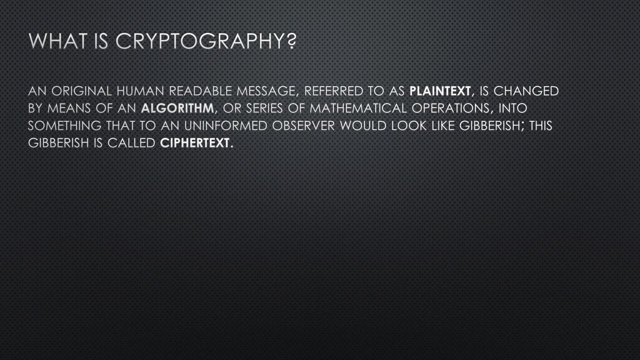 And part two, I'm going to focus more on symmetric cryptography, and part three: I'm going to focus on asymmetric cryptography. So let's talk about, then, exactly what cryptography is. So, first of all, a wise man once said that an original human readable message, referred to as plain text, can be changed by means of an algorithm or a series of mathematical operations into something that is basically, to an uninformed observer, would look complete gibberish. 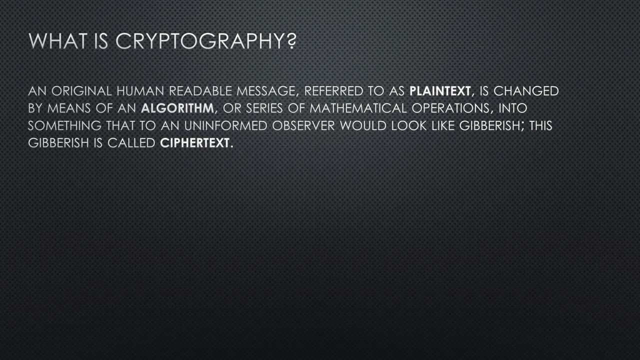 Now this gibberish, of course, would be called ciphertext, So plain text, of course, goes through the cryptography. It's a cryptographic algorithm and typically it involves the use of a key that only the sender and the receiver know about. 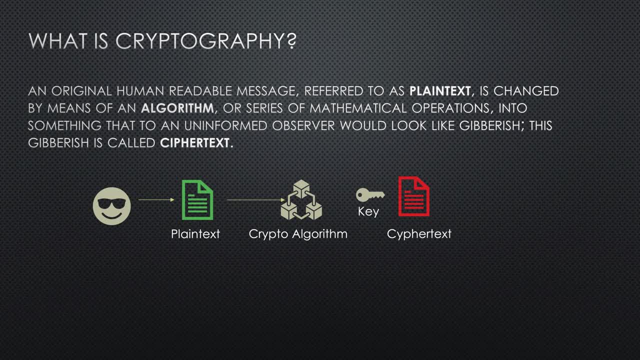 And, of course, if you don't have that key, then of course the ciphertext will mean nothing to you, unfortunately, So, of course. however, if you do have the key and you've got the right key, then of course we're on a winner. 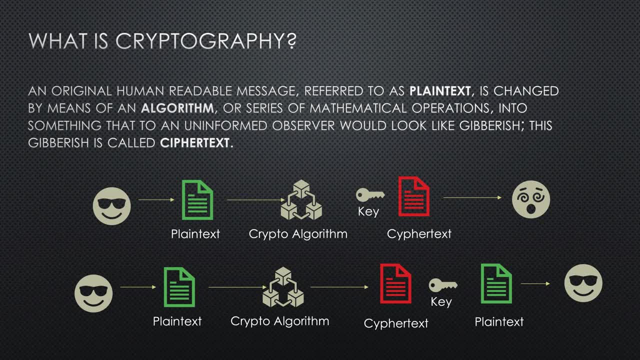 So again, cryptography was originally born out Of war, I suppose, the need to keep secrets, And, of course, it's nothing new: Cryptography is hundreds or thousands of years old actually. So why do we use cryptography today? 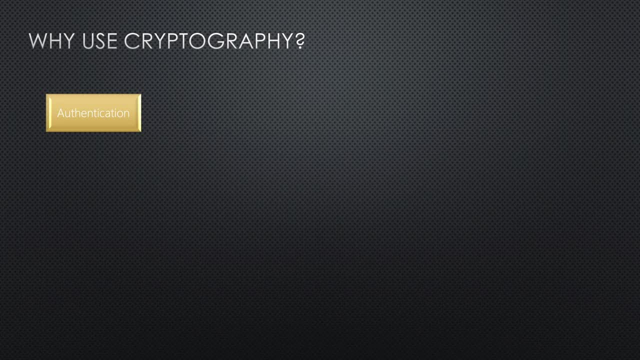 Well, we use it for a number of reasons. We use it for authentication, We use it for authorization, We use it to guarantee privacy and confidentiality. We also use it for integrity. That means, if I send you an email, you know that. 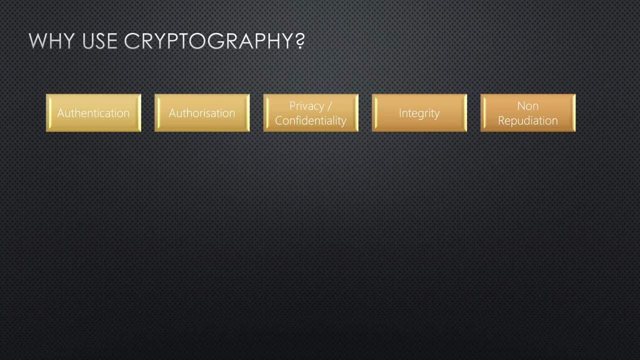 But this message hasn't been tampered with, and also non-repudiation. So you can't go to your bank account, take out 50 pounds and say I didn't get my money, No, you did get your money. So there's a whole bunch of reasons why this happens. 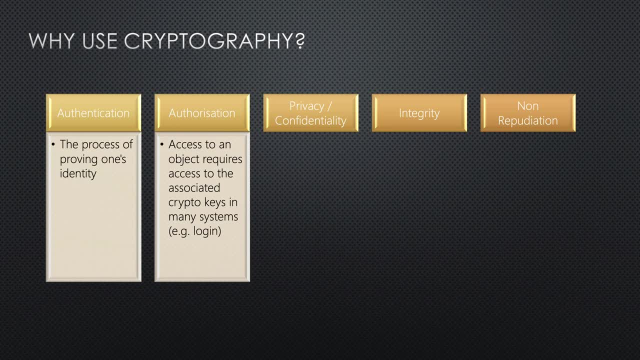 So authentication is the proving of one's identity. Now, of course, you go on vacation, If we ever get to go on vacation again. you have a passport And your passport. Your passport is issued by a trusted authority Authorization, So once you get into the airport, your airline ticket gets you through the security gates. 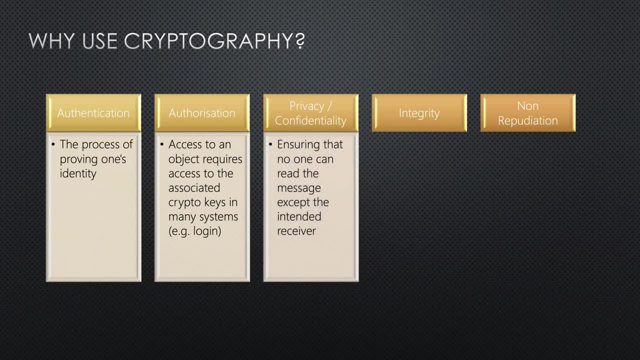 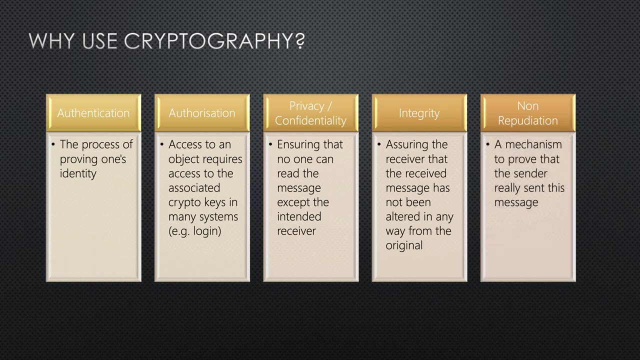 So that's your authorization to be there. Privacy and confidentiality, of course, means that no one can read the message except the intended receiver, And integrity. It ensures the receiver's message has not been tampered with in any way And non-repudiation, as I've mentioned, proves to the sender that he actually read the message. 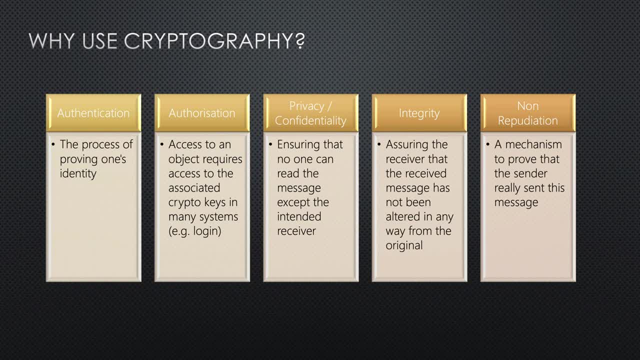 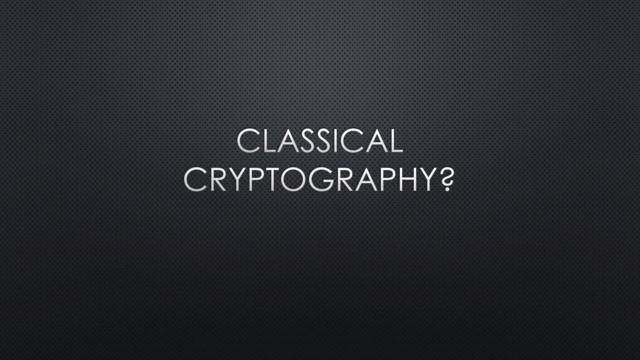 So, if you think about it- authentication, authorization and auditing- I suppose you would call that really Now, classical cryptography. as I mentioned, cryptography is something that's not new. We think of cryptography being something that we use every day, which we do. 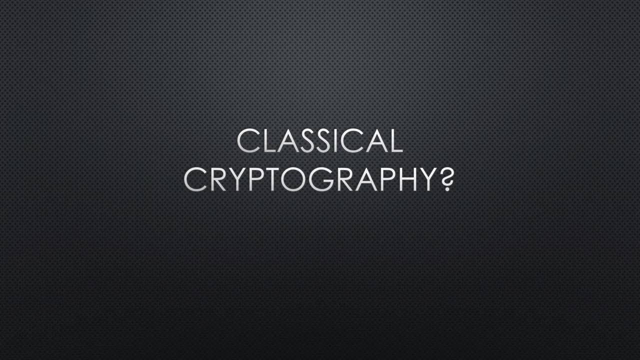 We use it on the Internet with our finances. We use it on financial transactions. We use it to keep our data safe on laptops or on PCs. For example, Microsoft BitLocker is based on AES encryption, But classical cryptography actually can be dated back thousands of years. 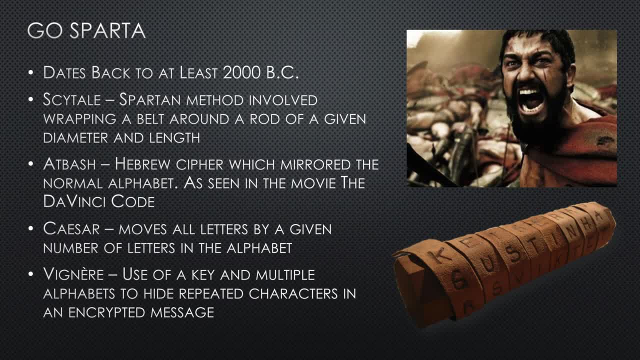 And, as you can see, it involves a large stick with a belt with symbols on it, And the idea was that, of course, the sender sent the rider with the belt when they got to the other side, The receiver. The receiver had exactly the same width and height of pole, wrapped the belt around the pole and read the message. 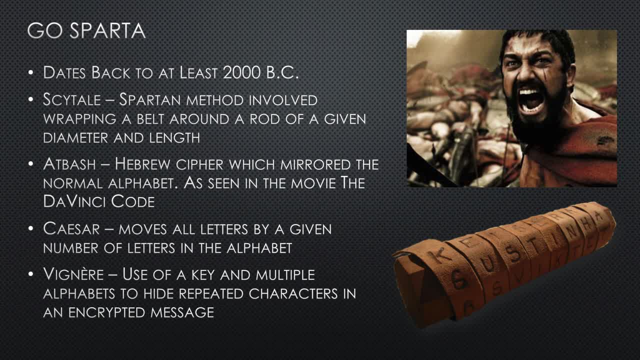 Another old method was something called at-bash. Now, this was an old Hebrew cipher which just essentially mirrored the normal alphabet, For example seen in the movie like the Da Vinci Code, for example. Caesar cipher, So Julius Caesar cipher- moves all the letters by a given number of letters. 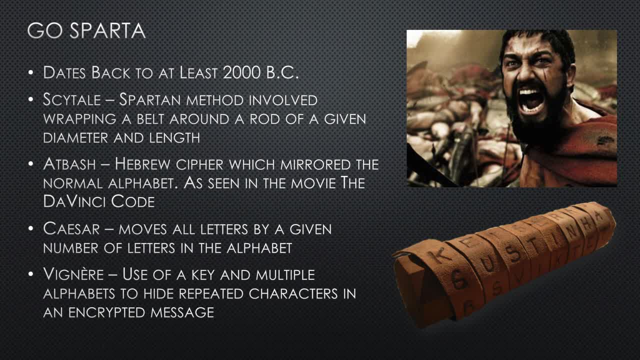 In the alphabet. So, for example, three characters: Visioneer, basically, was one of the first times that multiple ciphers were used, And this dated around to the 1500s and was actually developed by a man called Giovanni Bellasio. So let's take a look at some of these in more detail. 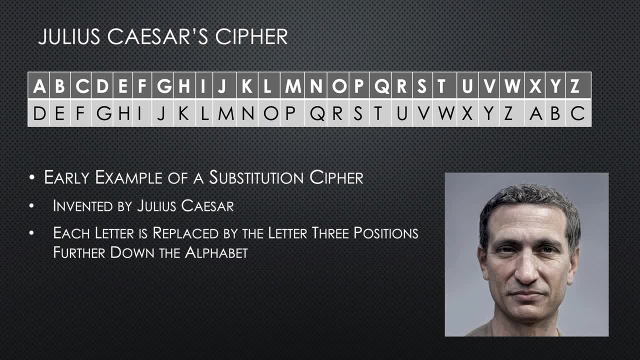 Julius Caesar. Now, actually, I was just doing some research the other day. This is actually a reconstructed face, using AI and a lot of hard work, of what Julius Caesar would actually look like today. Isn't that incredible? Anyway, this guy was a genius when it came to cryptography. 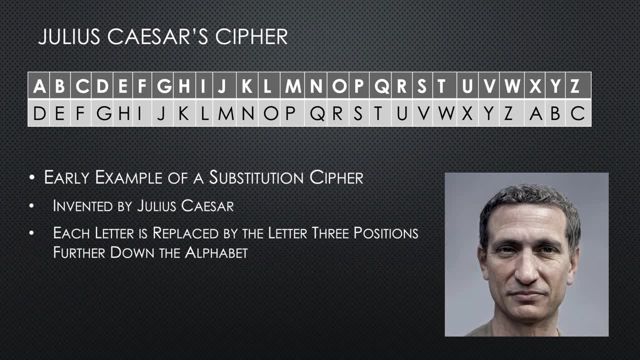 And he came up with a very early example of what we class as a substitution cipher. So a substitution cipher is a cipher that substitutes one character to another, And you can have a lot of fun with this. So, for example, A becomes D, B becomes E, C becomes F and so on. 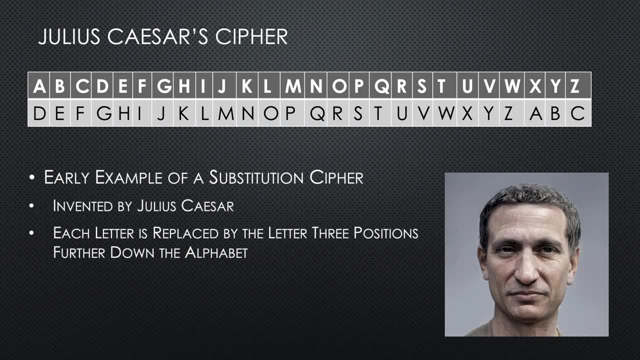 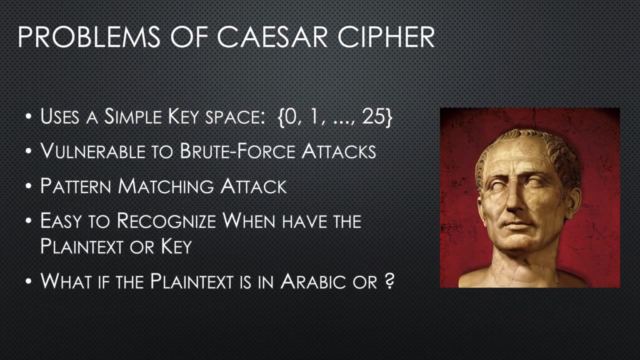 You just simply move the character, move the alphabet by a certain number of characters So invented by Julius Caesar. Thus the word cybercrime becomes. it becomes inconceivable, what it actually is. So, of course, the problems of Caesar cipher. 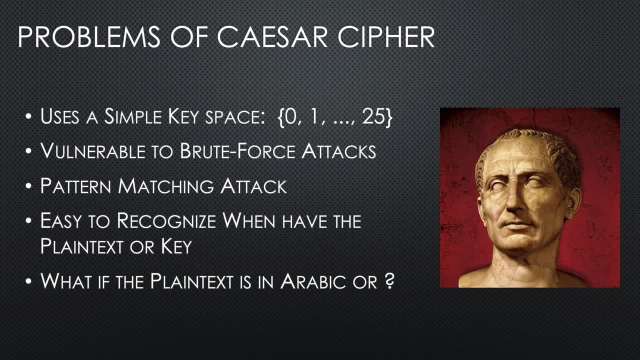 So, of course, the problems of Caesar cipher, So of course, the problems of Caesar cipher Is it uses a well-known key space, for example the alphabet, And of course this is potentially vulnerable to what we call a brute force attack. 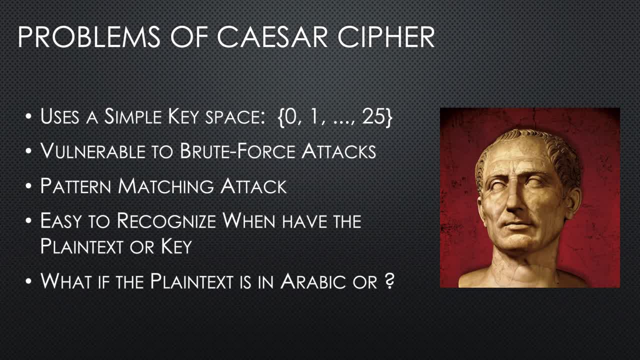 Now a brute force attack is essentially where you're trying. every single combination of characters, A scene, a famous scene in the movie War Games. If you've ever seen that War Games, the computer at the end is trying to launch the ballistic missiles. 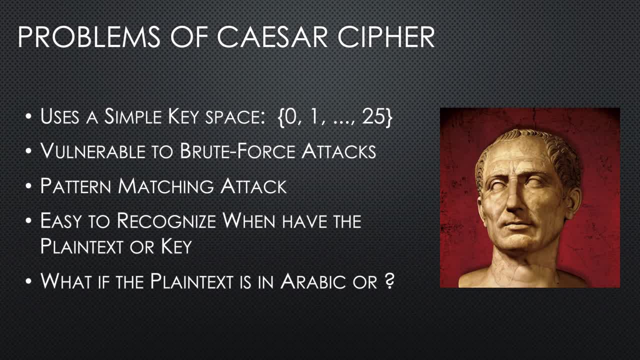 And he's going. He's trying every single combination of a launch code. Another type of attack is called a pattern matching attack, which I'll explain in a moment And again. of course, all of this is easy if you've actually got the plain text or the key. 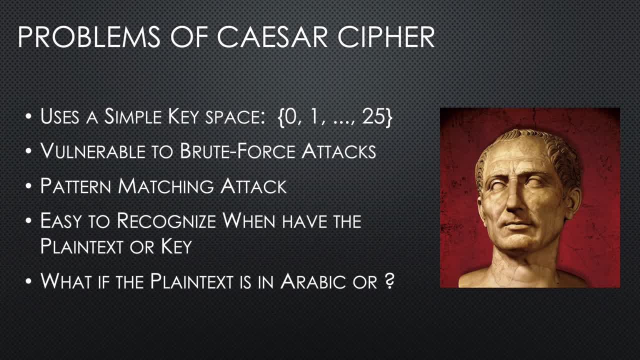 And the key in cryptography is the absolute most secret thing. So if your adversary knows the key, then it's essentially game over. Now I'm often asked: Ah, but what if the plain text, Andy, is in Arabic or Chinese or French or whatever? 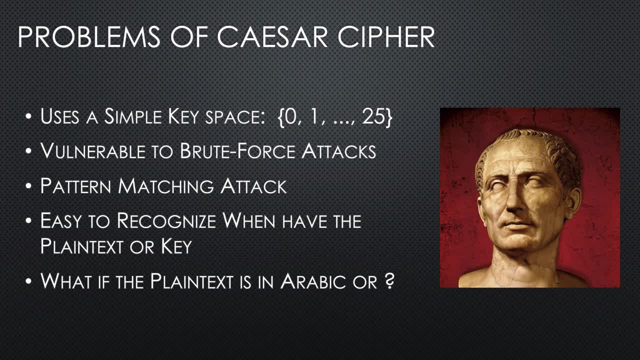 It doesn't really make any difference. It's because the language that we speak is rhythmic, It's pattern based, all human language. So if you think about a child, a baby, when they start learning language, they the first thing that they learn is something called phones. 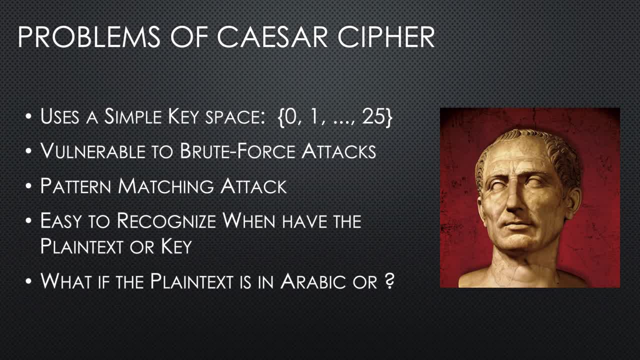 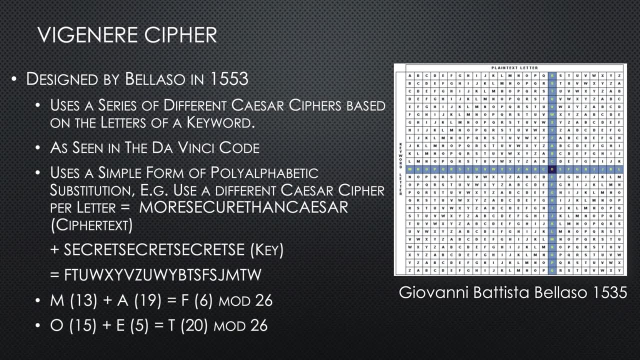 So ma ma, da, da, ba, ba, It's all patterns. Okay, So, visioneer, Now, as I said, Giovanni Bellagio in 1535 came up with something like this, And this was a massive leap forward in cryptography at the time. 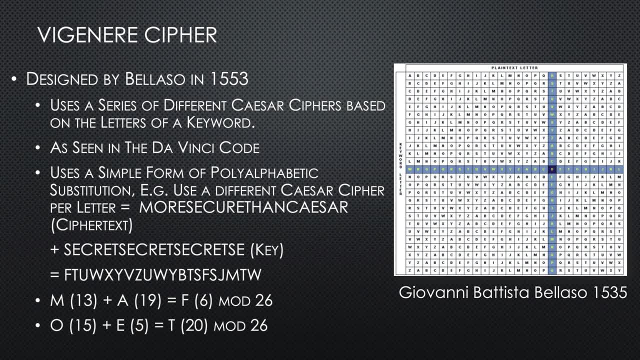 This was actually seen in the movie The Da Vinci Code And if you look closely you'll see. it's nothing more than men, In fact, numerous Caesar ciphers, And you can see, And you can see in both rows and columns. all the Caesar cipher is done is it's moved each row by one character. 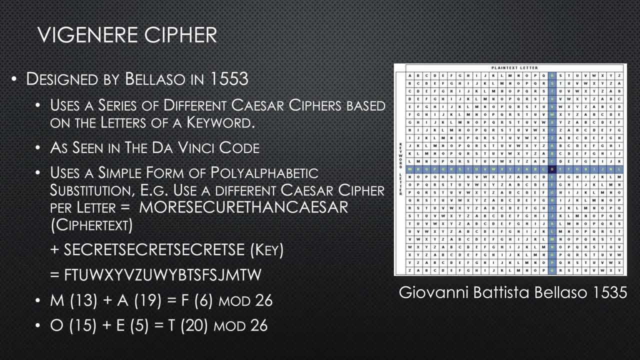 Now this is called a monolalphabetic Caesar cipher, In other words, multiple alphabets here. Now you can see. of course, the difference here is that the Caesar cipher just had 26 characters in the English language, But this has multiple, potentially millions of potential combinations. 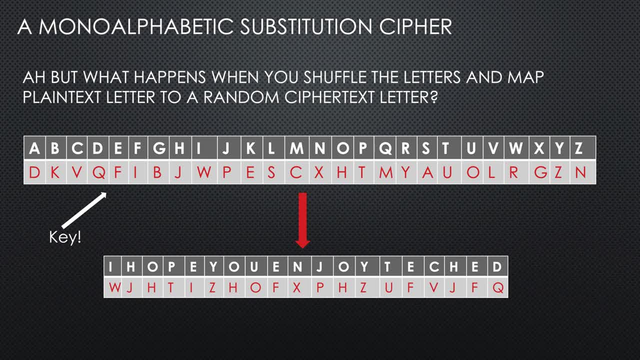 Okay, So a monolalphabetic substitution cipher. you could then say: ah, Andy, but what happens if you shovel? shuffle the letters? So don't use a pattern, Just throw them out there at random. Okay, What about that? 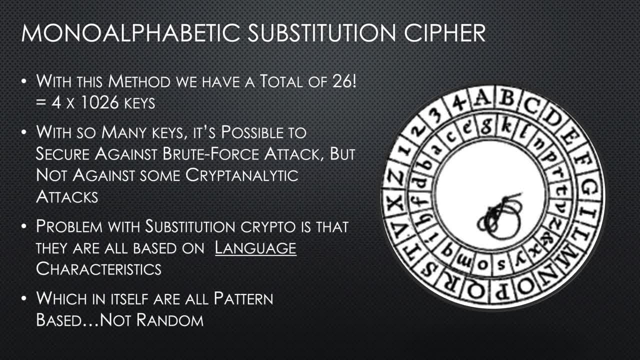 Well, okay, Fair enough. Yes, Okay, That would still increase the number of potential keys, However you can. it would secure against brute force attack, but not against some crypto analytic attacks, And the problem is because this cryptography is all based on human language. 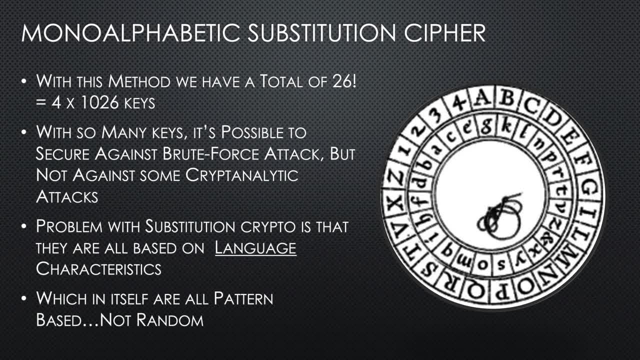 And again, human language. if you've ever seen the movie Jurassic Park, remember Jeff Goldblum's pattern. There's no Jeff Goldblum's seen, rather There's no such thing as as random. His argument was that everything in humanity is has a as a pattern. 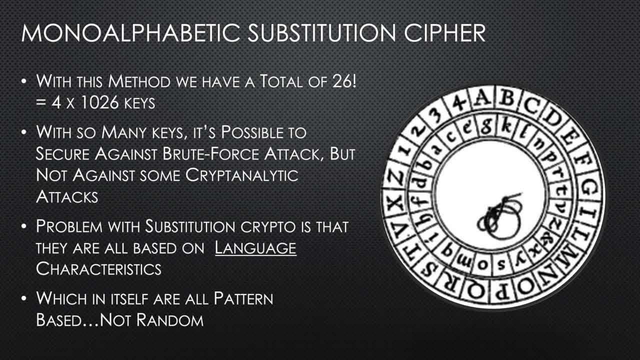 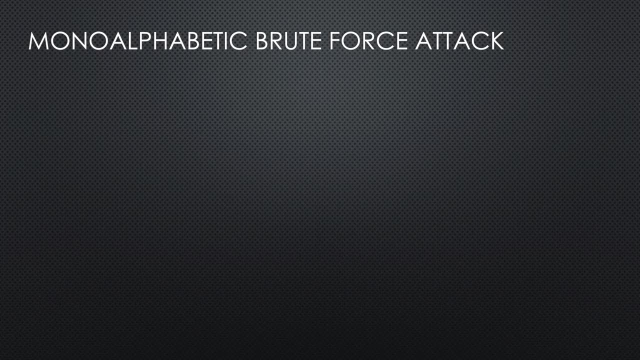 So there are seven days in the week, We have seven continents on the planet earth. You know, winter follows autumn, summer follows spring, and so on. It's all pattern based And it's an interesting concept. So monalphabetic brute force attack, then, would basically work like this: 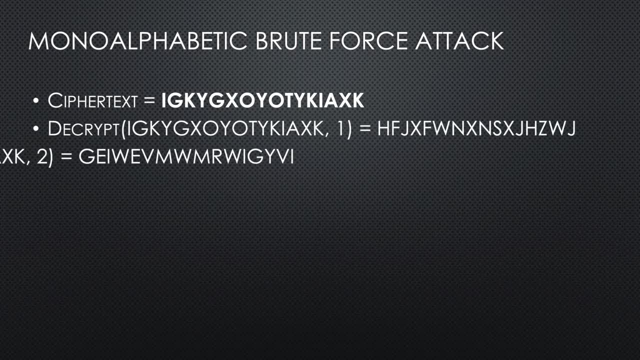 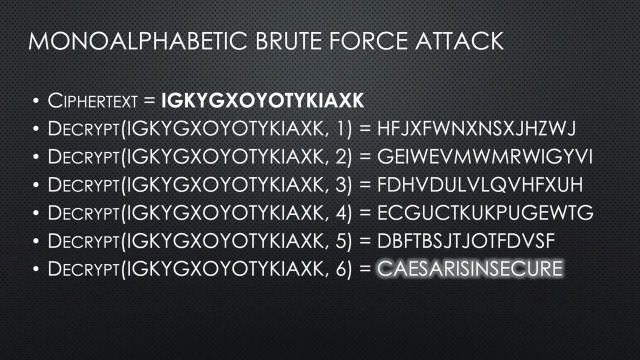 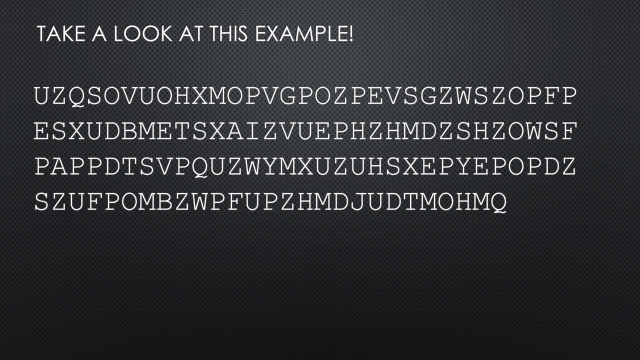 So, basically, you're trying every single combination And eventually, of course, you work out that, yes, there is a pattern here. Now here's a question for you. Take a look at this early, this very, very simple example- And this was a real world message from the 1970s, by the way. 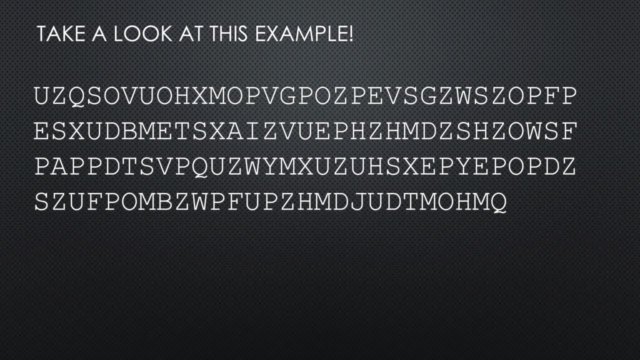 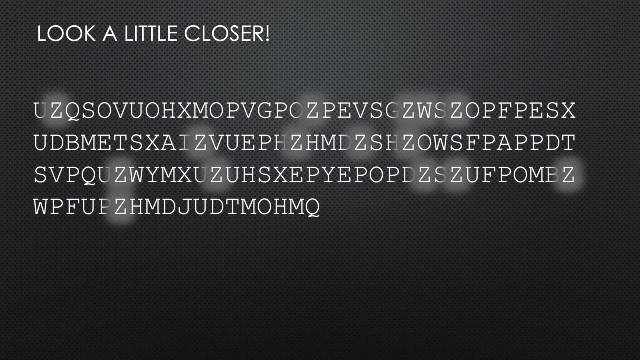 Now, when we talk about pattern matching, look at the characters here. What are the first things that leap out? So there are some letters here that appear more than anything else. Let me start you off The zeds. There's an awful lot of zeds in this message, don't you think? 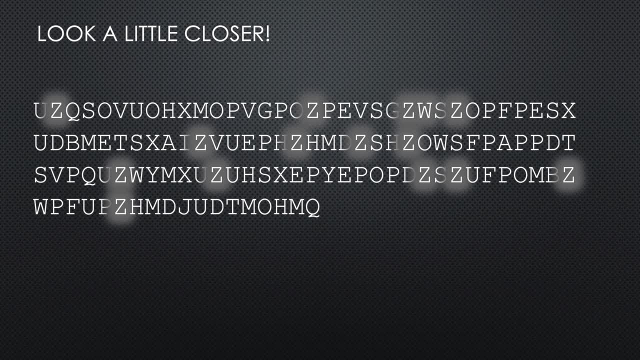 And if you look closer to the zeds, there are in a couple of places- in fact two or three places here, Where zed is combined with another character. So, for example, ZW appears a number of times. That's got to mean something. 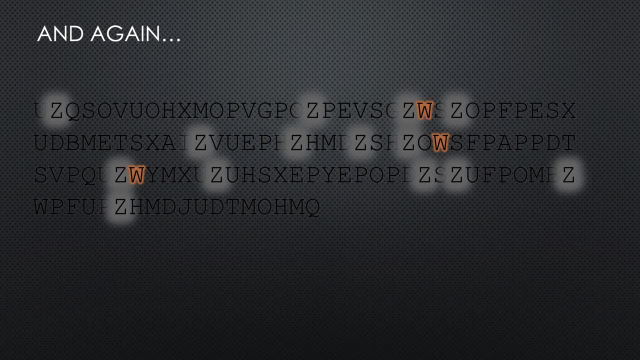 Yes, so you can see ZW, ZW. Okay, Again, some other letters, Q and U, S's, appear a lot. And what else have we got? A lot of O's, A lot of P's and so on. 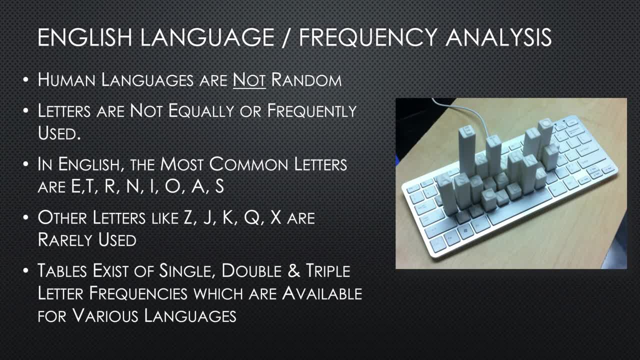 Now it's interesting. I don't know if you've played Scrabble, But if you've ever played Scrabble it's really interesting because those are the characters that you get most points for. Those are the least used characters. So when we go back to this you can see it's full of least used characters. 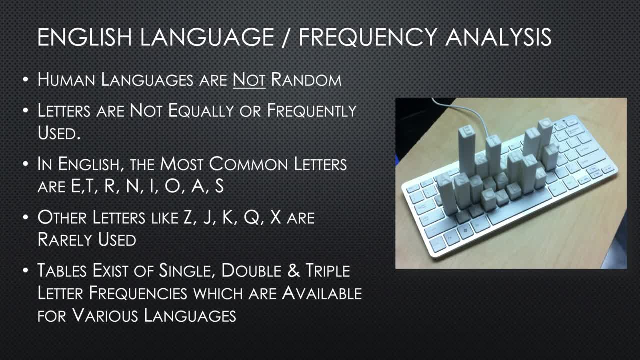 So with pattern matching, in human or in English language, the most common letters are ETRONIAS. So you see? So all we start to do is then think about: hey, well, what if we replaced those other characters with these? Well, surely in that case we could potentially work it out. 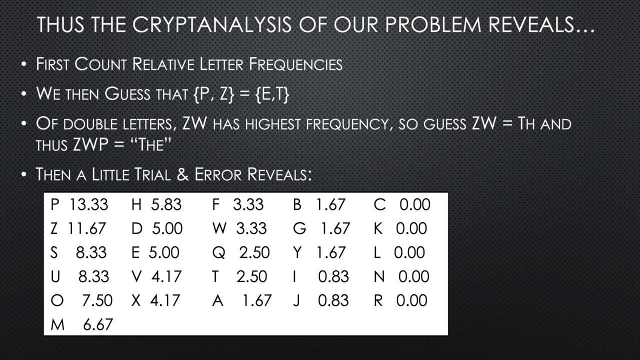 And this is essentially called a cryptoanalysis. Okay, So we work out that essentially, P and Z could potentially be E and T And, as we said, Z and W. So one of the most common words or most common sounds in English is TH. 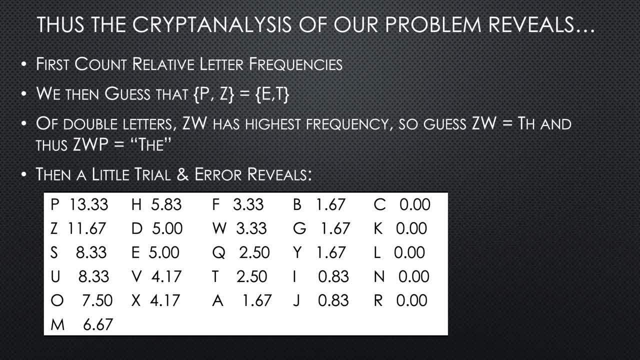 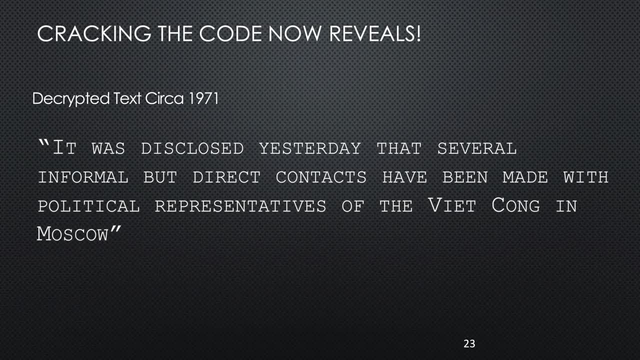 TH. So you can see ZW could mean TH. So thus a little work And we realize that this is what the message actually meant. Okay, This is decrypted text from 1971, from the Vietnam War. So from classical cryptography we move forward in time. 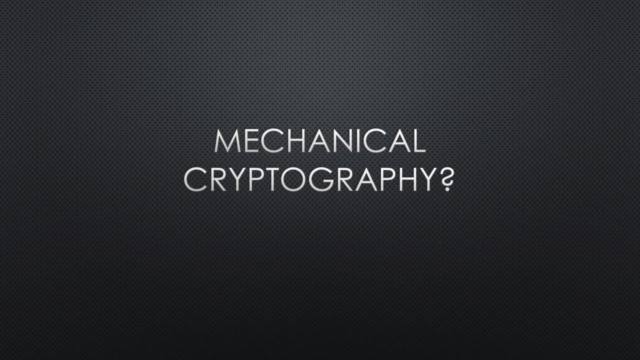 And, of course, one of the problems with classical cryptography is it's full of patterns. So no matter which pattern you love, I live in Scotland here. Mary Queen of Scots had her own cryptographic algorithm so that she could hide from the English. So now we come to the mechanical era and the mechanical era. 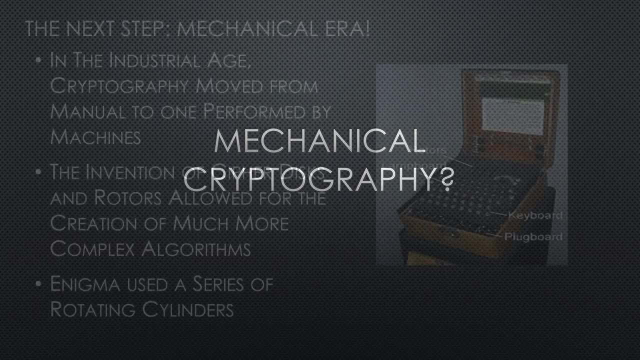 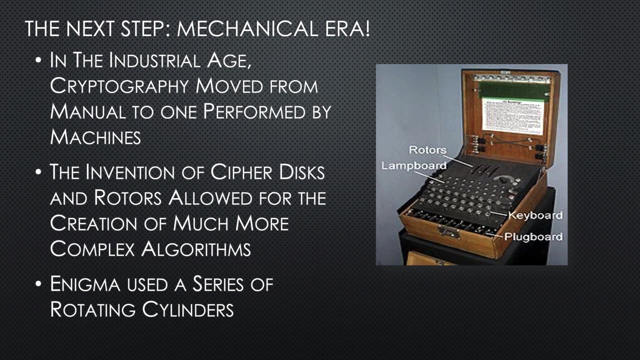 We cannot talk about mechanics without talking about the Enigma machine. Now, the Enigma machine here really is An amazing or was an absolutely amazing invention. So essentially what we have is: we have this machine here that's comprised of rotors, a lamp board, a keyboard and a plug board. 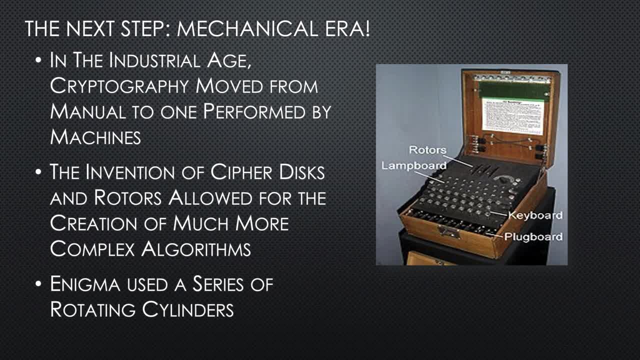 And the idea was that once you set this every day, every day at midnight, the code would change And, of course, the German officer that used this would set this the second time. Okay, And that's how you set the settings every day. 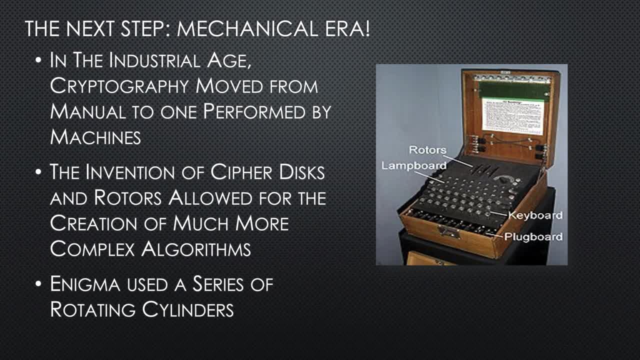 So even if you worked out what the settings were, it would change. And the clever thing is as well: every time you press So, for example, on a typewriter, on a QWERTY keyboard, you just press the letter A and it will go A, A, A, A A. 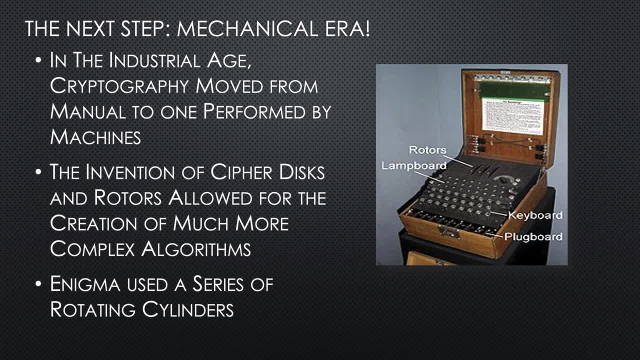 You press it on an Enigma machine and it goes and it will rotate the wheel, So it will go A, B, C, D, E, F just by pressing one key. And you can imagine that if you started typing a letter it would be almost impossible to work out what that is. 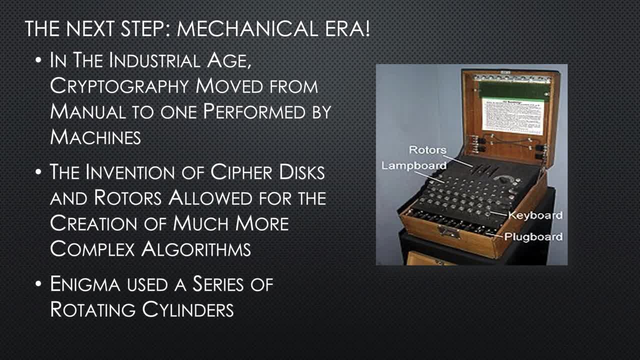 And this is actually another type of cryptography. In fact, this does a couple of different things. It doesn't just do substitution, So it substitutes something for something else, But it also does confusion as well, And confusion and substitution equals very strong. 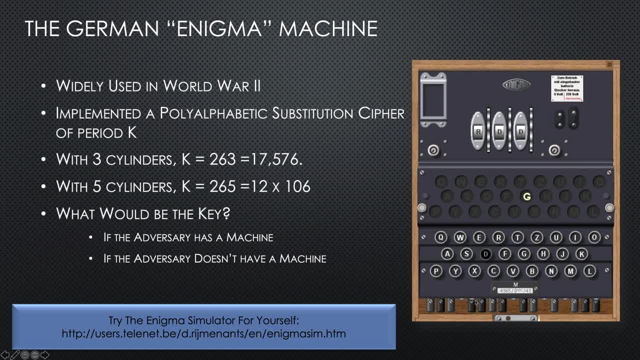 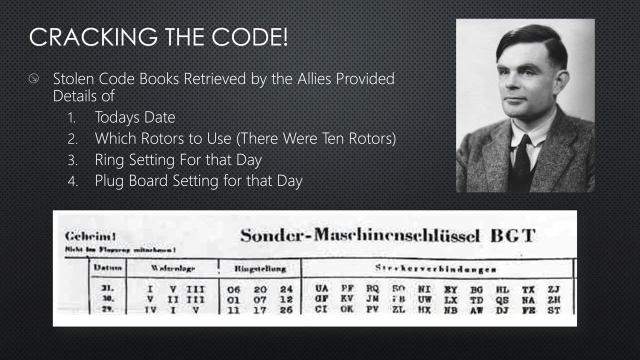 Cryptography. Now, in fact, you can actually try a simulation of the Enigma machine yourself. There are a number of places where you can try it. So how did it work? Well, as you can see, here is a copy of the German, or a German code book: here. 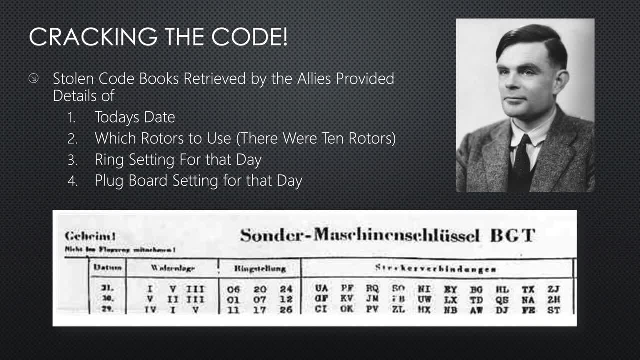 And it comprised of today's dates, which rotors to use Now in all the movies. by the way, if you've ever seen the spies working one of these machines, the interesting thing is that they're always in a room on their own. 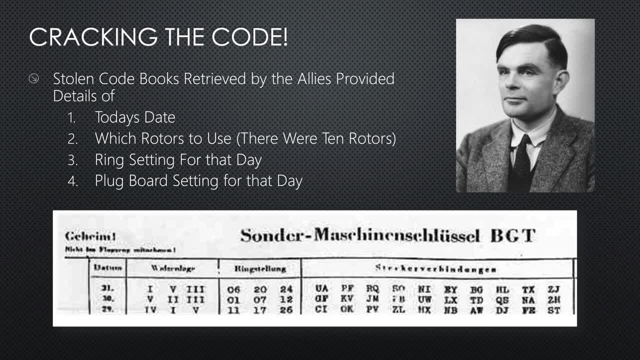 In reality, ladies and gentlemen, that would never happen. You actually needed about three people to work an Enigma machine, And there were different versions as well. So, for example, there was a three ring version: for the military, for the army. 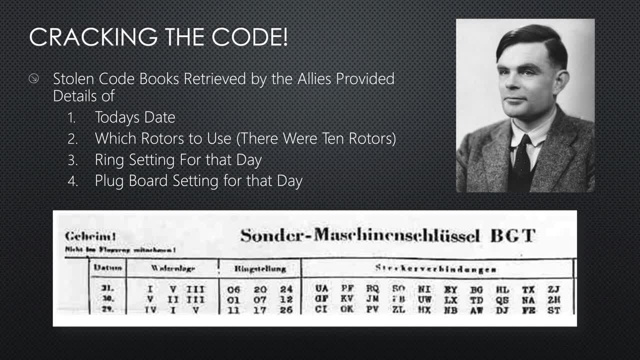 There was a five ring version for the submarines, There was another version for the Air Force, and so on, And, of course, the allies also had their own version of Enigma as well, And it was this man, Alan Turing, of course, that eventually cracked the Enigma code. 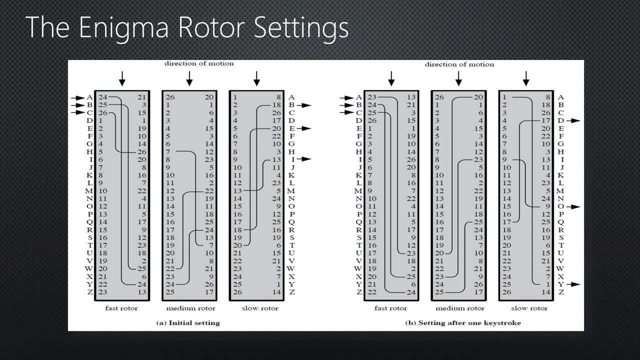 as seen in the movie The Imitation Game And, as you can see, the Enigma rotor settings. And the clever thing is you change the rotor settings and the plug board and lamp board settings every day at midnight And therefore you know if you didn't have the code, if you didn't have those settings. 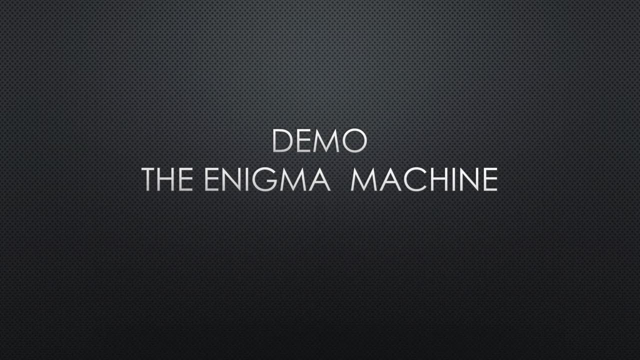 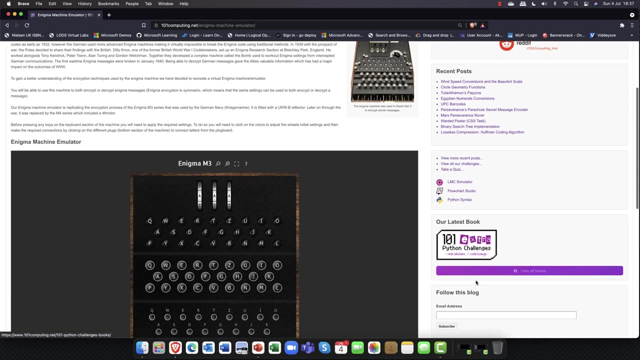 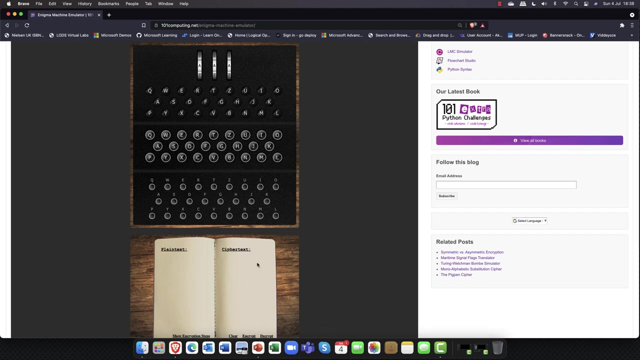 then you would not be able to read the message. Now, as I mentioned, you can try the Enigma code machine for yourself. There are a number of different emulators here And you can see that this is one here And we've got the plain text on the right hand side here. 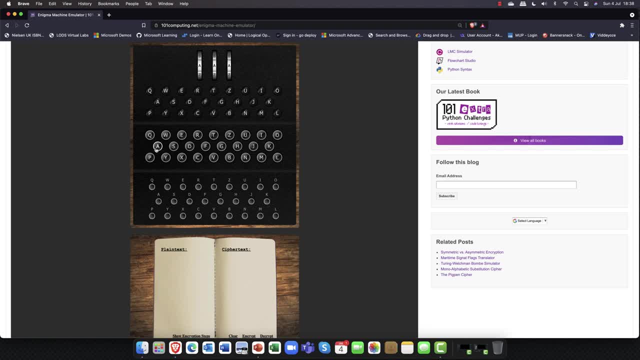 And we've got the ciphertext here Now, just straight out of the box here. If I just start pressing the letter A, you can see it starts rotating And you can imagine if I was typing. you know I'll press a spacebar. 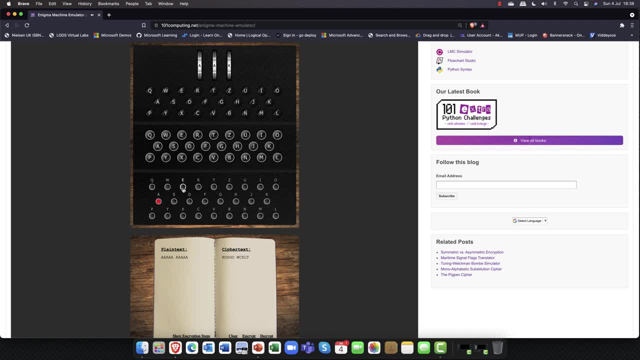 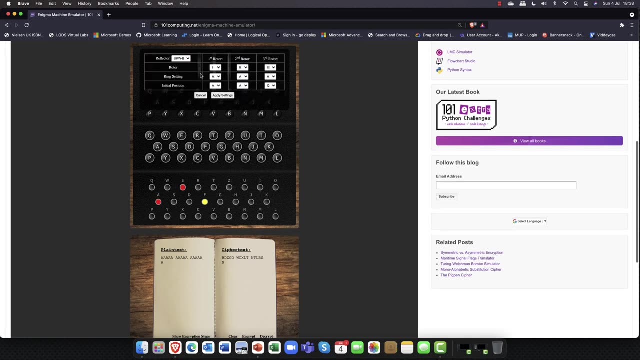 And look what happens if I change the lamp board settings. So once you start changing things, you can see it changes it even further And you can imagine Again. I could change the word, I could change the wheels, I could change the different characters here. 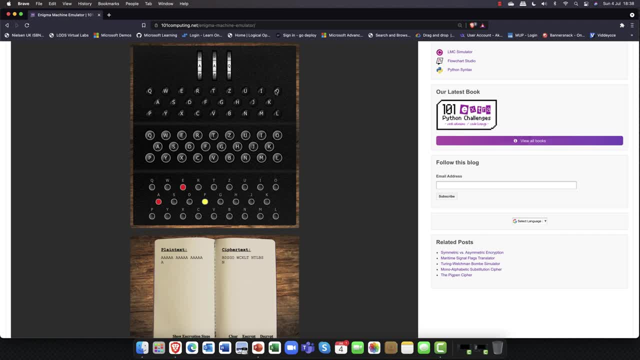 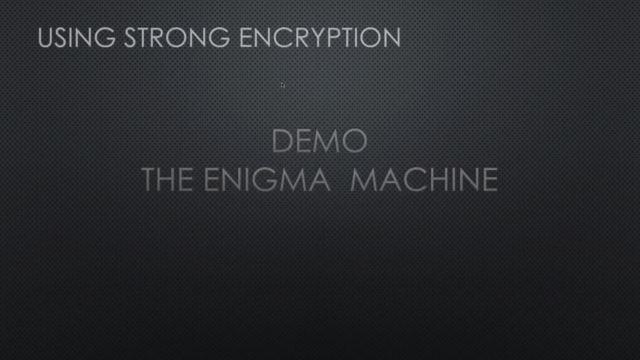 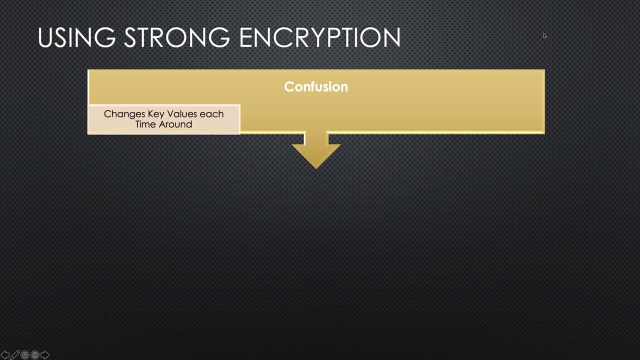 So this in its day almost won Germany the war. Absolutely brilliant technology. So try it out yourself. It's a lot of fun. So when we talk about strong encryption, I mentioned that it's a combination of confusion, And confusion changes the key values each time around. 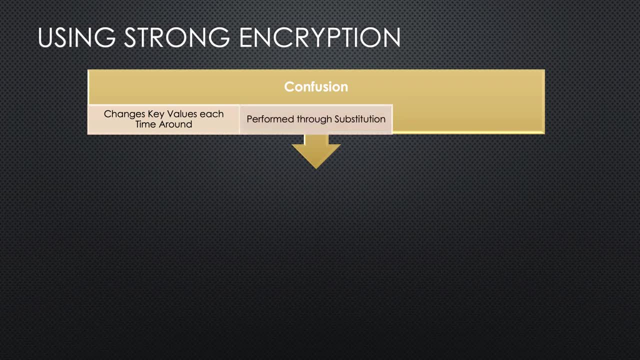 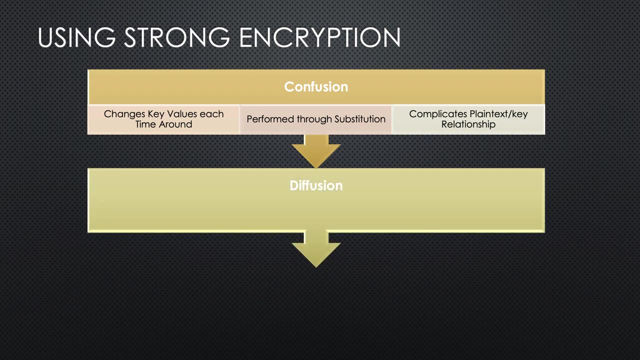 So you saw it in CaesarText. It's more so in the Enigma code machine, And this is performed through substitution And it complicates the plain text. crypto text relationship Diffusion, on the other hand, changes the location of the plain text in ciphertext. 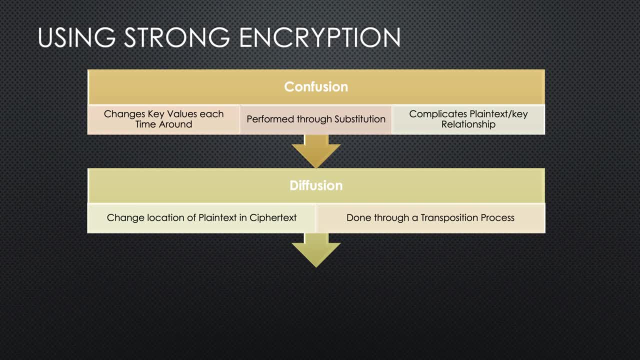 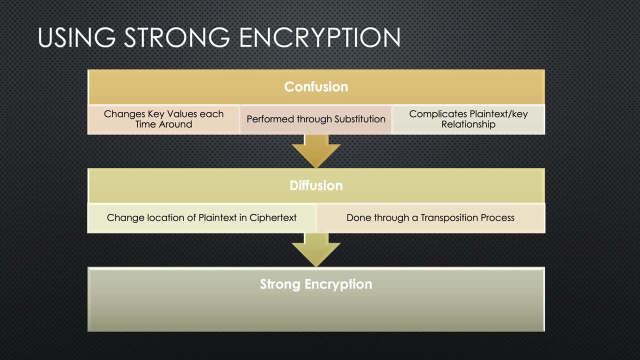 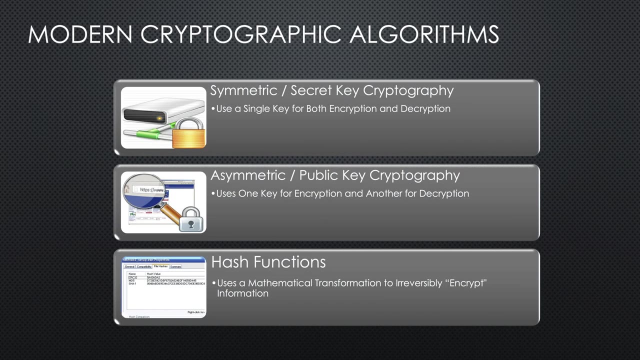 And this is done through something called transposition. So this is where you're changing one character around. You're moving the characters around. So this together equals strong encryption. Okay, Now, when we come to modern cryptography, really there and again, this is an overview. 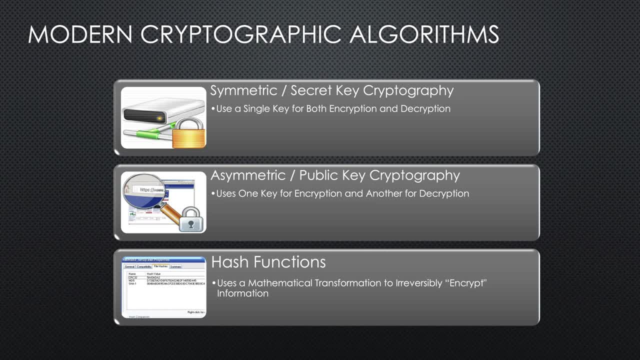 Do remember that, And we're going to look at this in future sessions together. So when we talk about symmetric key cryptography, this really just uses a single key. So a single key, And this is great for things like large Volumes of data. 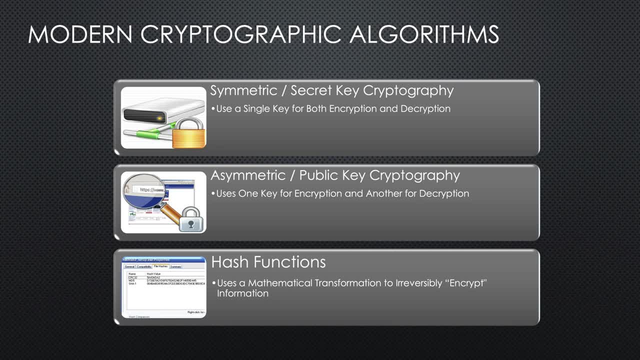 So your hard drive, for example. So if you've got a, let's say, a Windows 10 laptop, you can encrypt the hard drive with BitLocker, And BitLocker uses AES encryption, And AES encryption is an symmetric algorithm. Asymmetric cryptography, on the other hand, uses two keys. 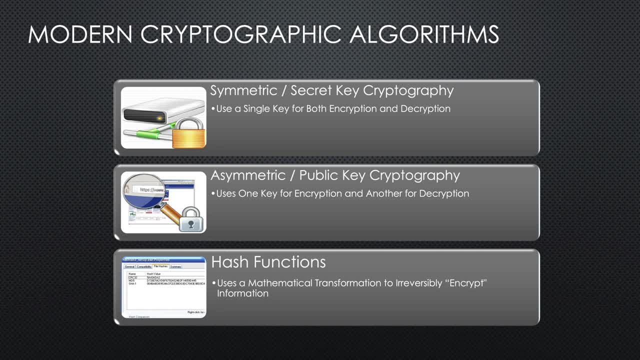 It uses a private key and a public key. So, for example, if I'm sending a message to you, I know your email address, That's your public key, So I send the message and I encrypt it with my private key. So when you receive the email, you're getting the email from my public address. 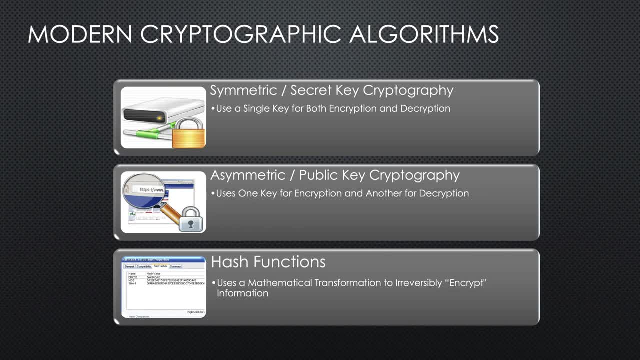 And you can see that it's coming from me. But you can open the message with your private key. See what I mean: Public private key. Also, hash functions are very useful as well. Hash functions provide integrity Because they use a one-way transformation process. 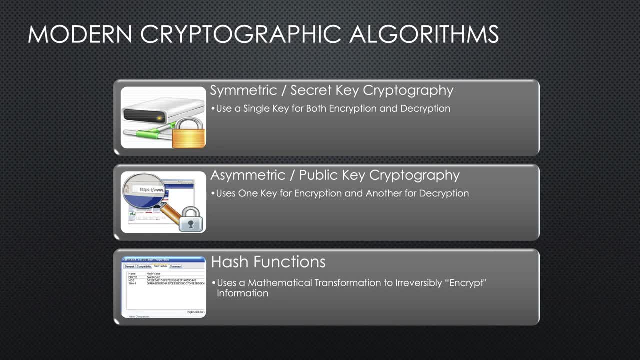 And what this does is irrelevant of the amount of data, So it could be the Encyclopedia Britannica, Or it could just be a few lines of text. It produces the same output size. Okay, And it's absolutely brilliant. And the idea is that if I sent you a file, 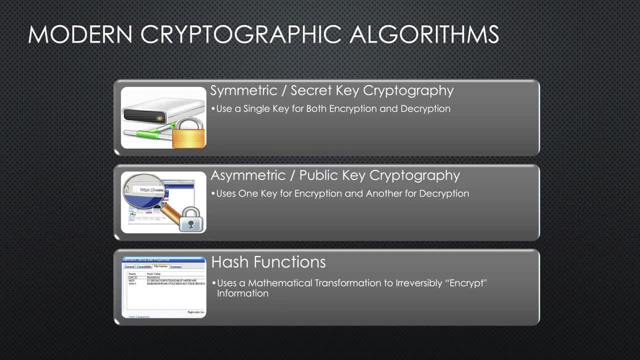 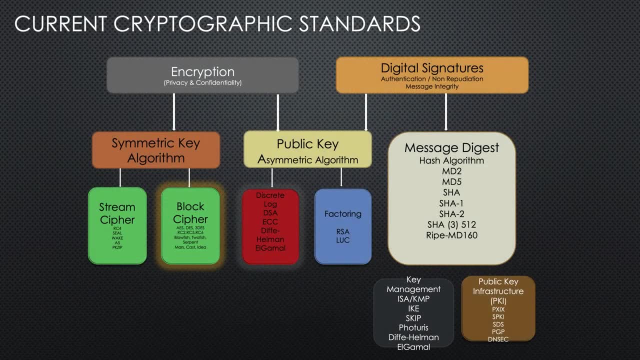 And that file's hash value Was different to what you were expecting. You know that that's been intercepted and changed. Now there are lots of different cryptographic standards And, as I said, in future sessions We're going to look at these in more detail. 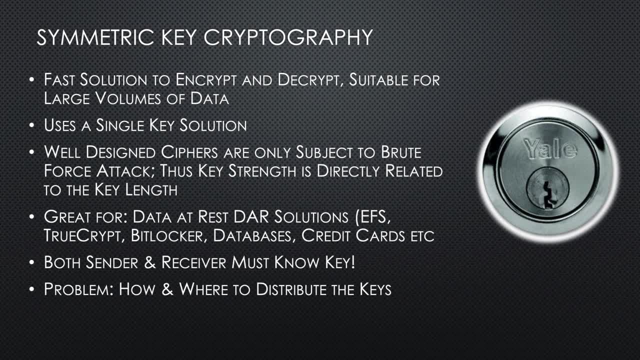 Now, symmetric key to cryptography is brilliant. It uses a single key, It's fast, It's efficient And it's great for very large volumes. But, of course, like any cryptography, Where do we store the keys? That's the thing. 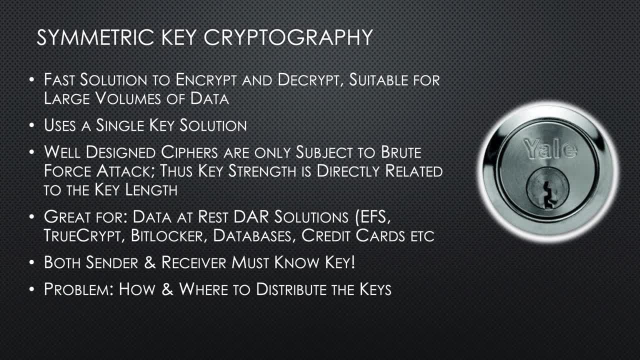 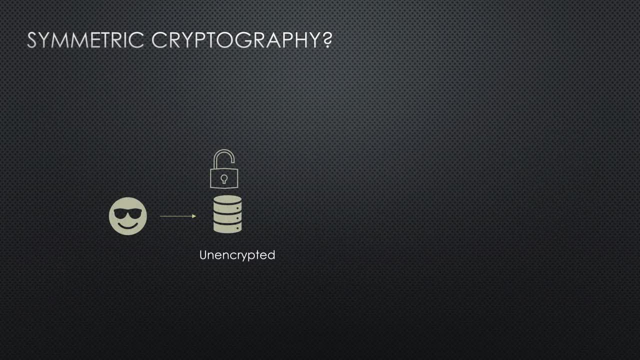 And, of course, like all cryptography, You have to keep it, you know, private, And that's the key thing. Okay, So symmetric cryptography- Fantastic for large volumes of data. So I encrypt the data with my symmetric key And, of course, once it's encrypted, 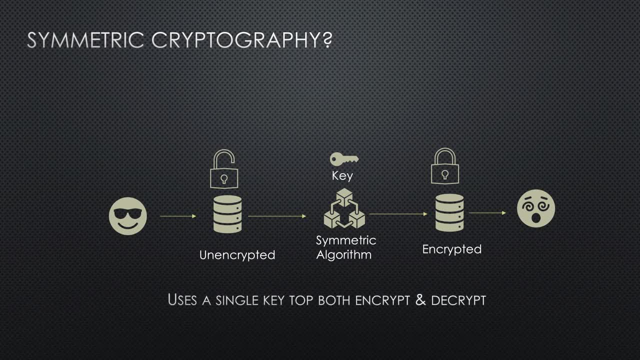 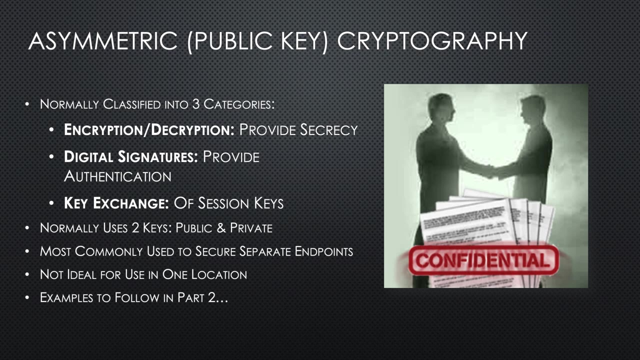 If you're trying to get access, Then you've got no chance. So the key thing here is it uses that single key For both encryption and decryption. Okay, And again examples: BitLocker and AES- Okay, So asymmetric cryptography. on the other hand, 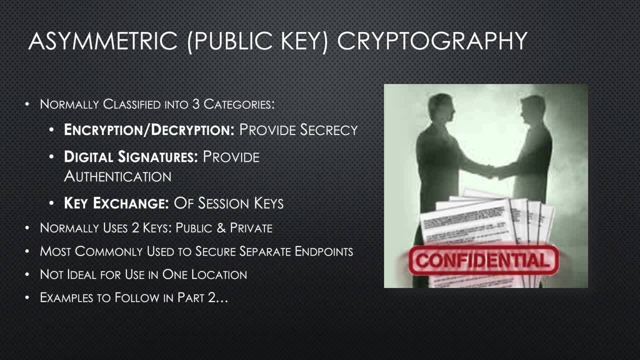 Normally used for a number of different areas. So encryption and decryption. It can provide something called digital signatures, It can be used for authentication purposes And you can also do what we call a key exchange. So, for example, if you're buying items on the internet, 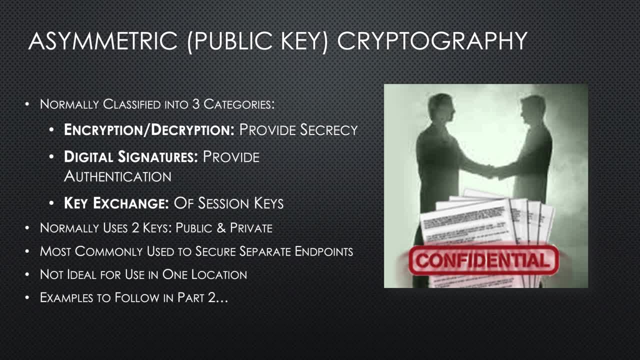 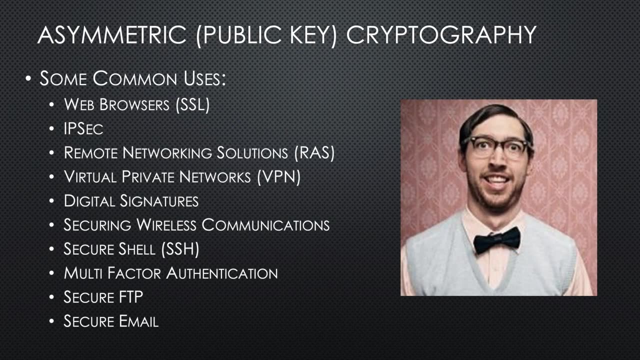 For example, Again because it uses public private key, Again it's not ideal for use in any one location And again we're going to show you this in much more detail In a future session. So, asymmetric or public key cryptography. 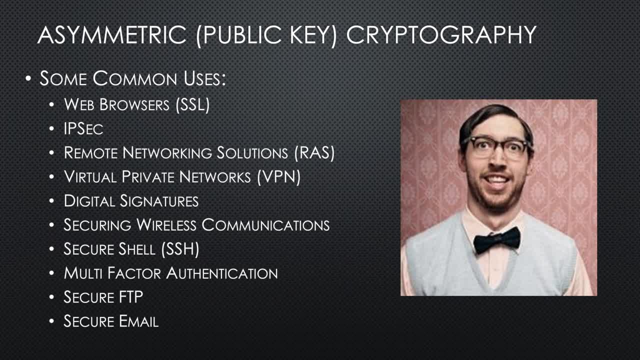 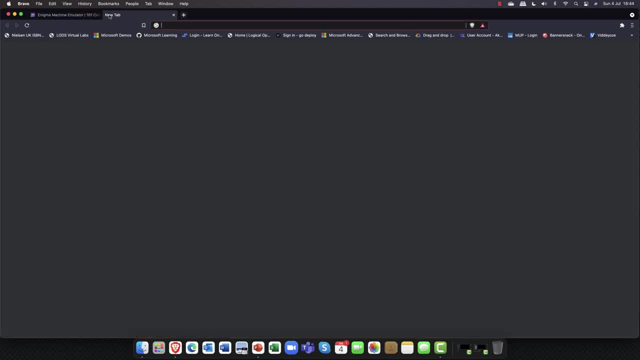 You can see this every day. So if we go back to our web browser, And in our web browser up here, You can see that the Let's say, for example, I go to Google, So, or Amazon or Microsoft, So if I go to 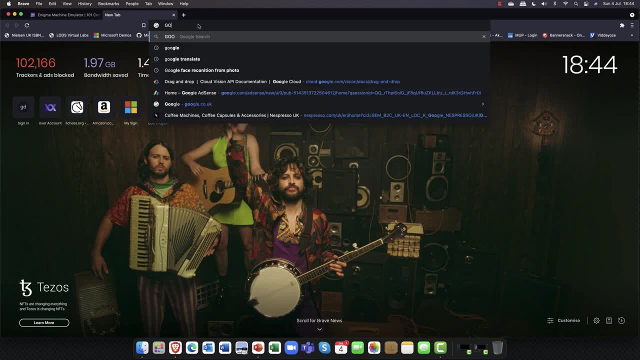 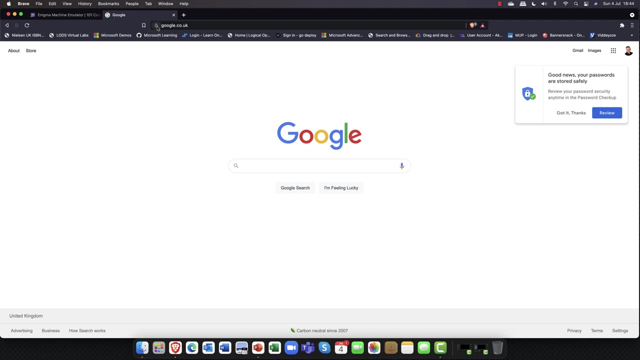 Let's say my Google page. Sorry, just type this in: So, Yes, Okay, So Google, There we go, There we go. So you can see that up here. We have this padlock up here And this padlock shows me that my connection is secure. 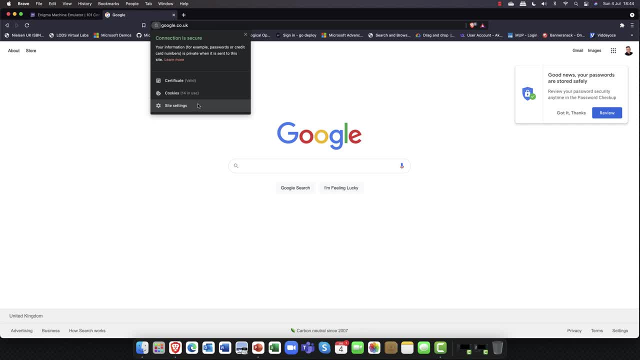 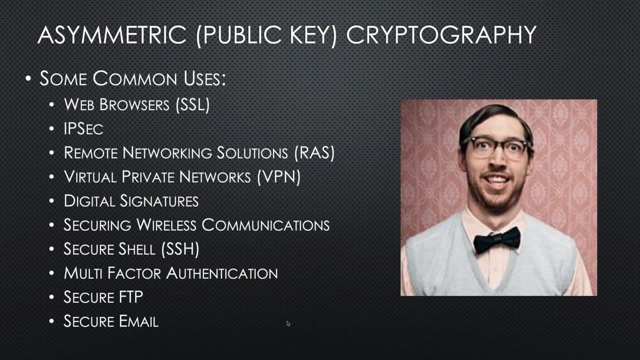 And now, just how exactly does this work? Well, again, this is something I'm going to go into A nice deep dive in that future session. All right, So other things that it can do: It can provide things like Remote networking solutions. 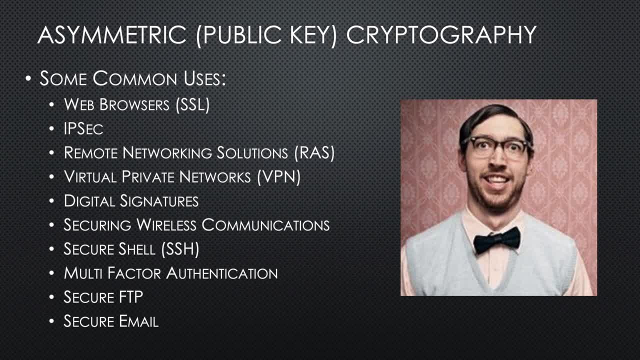 Virtual private networks. So that means that you can tunnel Through a private network, through the internet. So, for example, If you're in Starbucks and you need to Do some work inside your company Headquarters, Then you can tunnel through your company headquarters. 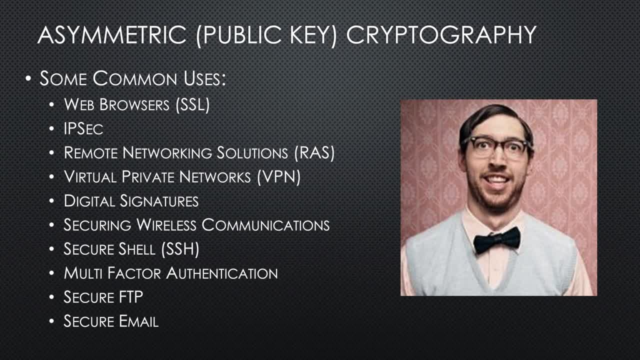 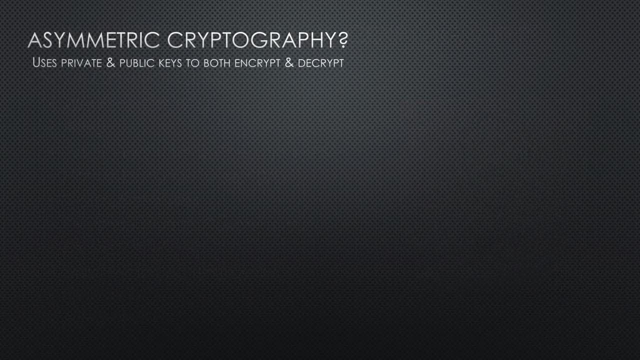 Using the public internet File transfer, Secure email and so on. These are all technologies That use public private key Cryptography. So essentially what happens here? The sender encrypts the data With their private key, And I know it's going to you. 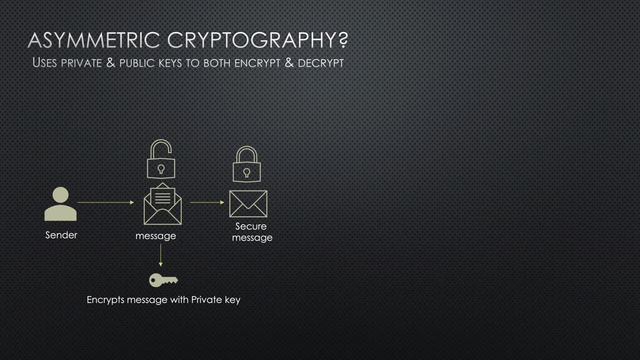 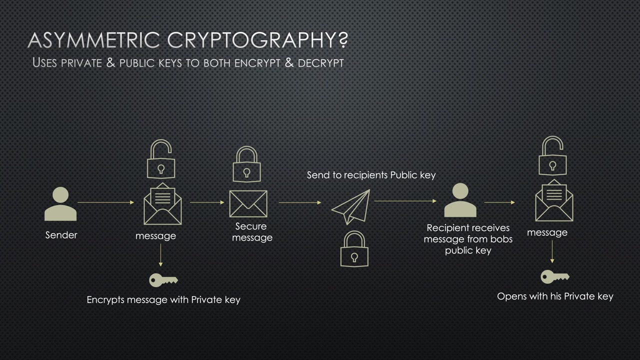 Because That message is now secure And I'm sending it to your public key, So your email address, Let's say So. when you receive the message, You can see that it's coming from my public key, But you unlock the message. 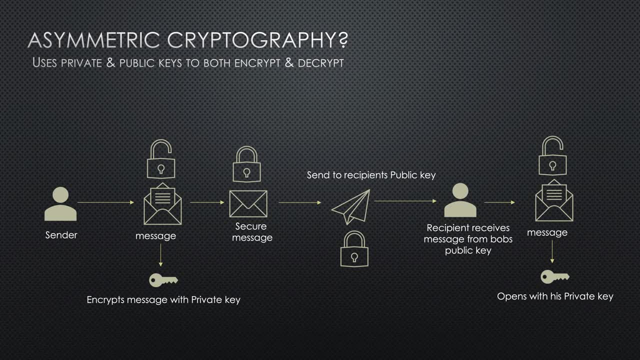 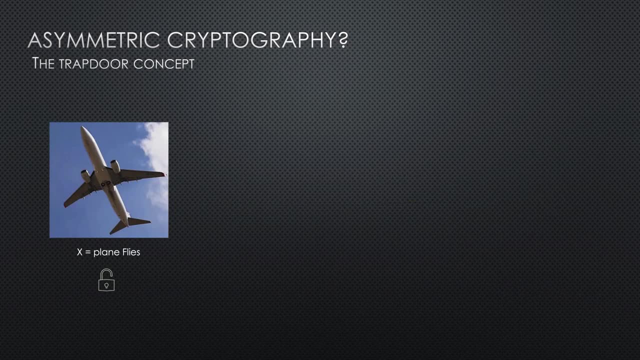 Using your private key. Thus, the contents of that message Are absolutely secure. So, again, Make it simple. So one of the technologies That made this really, really Easy to understand Was developed by two gentlemen: Martin Whitfield, Diffie. 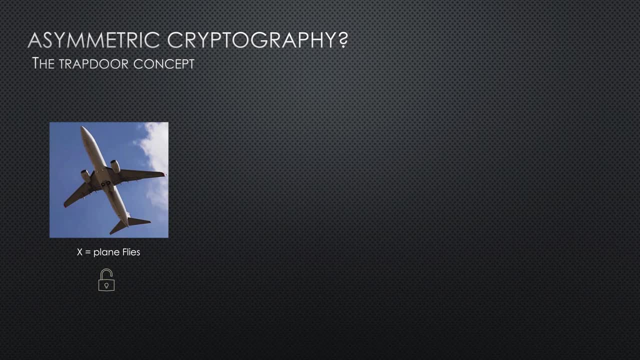 And Martin Hellman And they came up with something called The Diffie Hellman algorithm And it was amazingly simple. So they came up with this formula That says X. So if X- We know that a plane flies- We can see that the plane is flying. 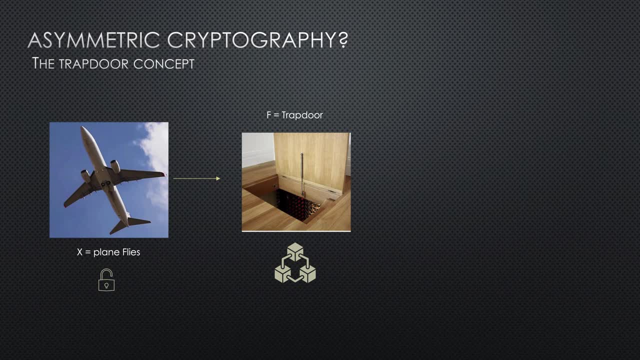 And they came up with something called The trapdoor function. And the trapdoor function Is it's easy to see Exactly how it works. So everybody knows How it works And it's you know, It's easy to see. X. 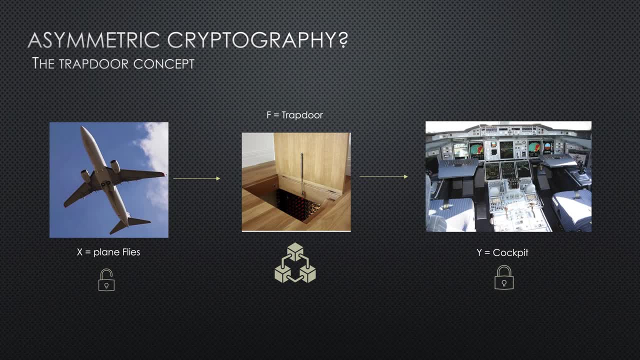 But It's almost impossible To reproduce it If you don't have the skill set. So X is the public key, Y is the private key, Okay, And F is the trapdoor function. So Y equals F Over X. 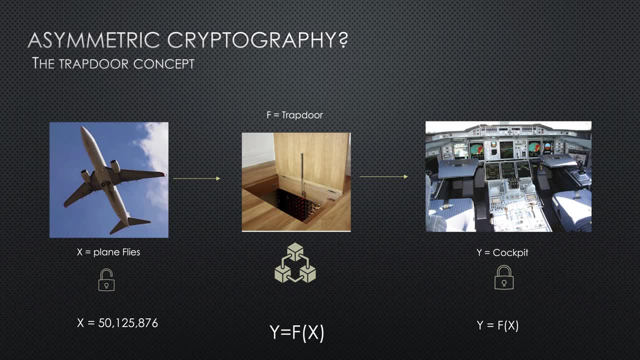 So it's almost impossible To work out What Y would be With that. one way Trapdoor function, And that is the cornerstone Of how we communicate On the internet Today. Now the final Piece of cryptography That I want to talk about. 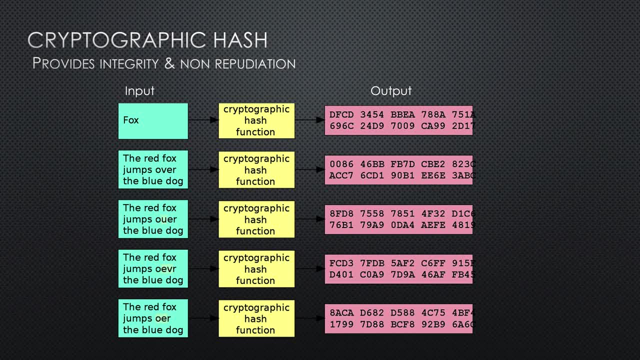 Is something called a hash value. Now, a hash value produces something called A hexadecimal. A hash value, Now a hexadecimal, is in 16 bits And, As you can see here, If I type the word fox, You can see And it runs it through the hash function. 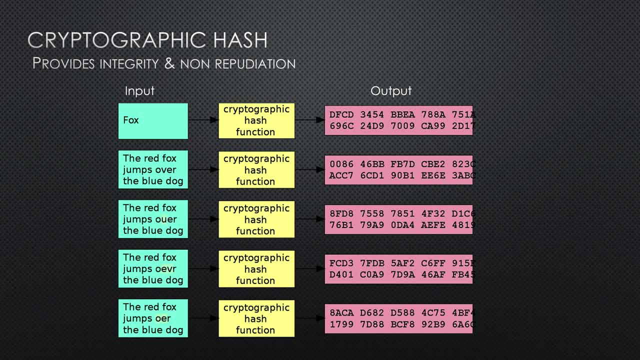 You get a specific output. If I add a piece of text, The red fox jumps. You can see the size of the output Does not change, But the content Of it does change, And you can see That if I change just one. 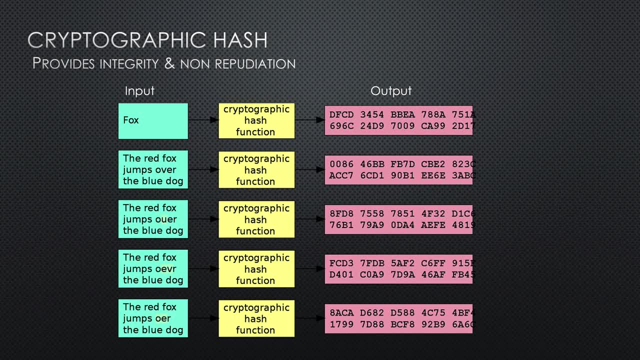 Character in that message. Again, the output Changes. So, from an integrity Perspective, If somebody had managed to Get hold of your secret message, You would know about it. So this is the cornerstone Of what this means, by the way, 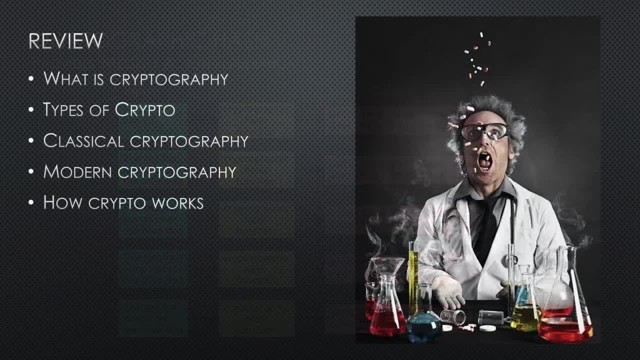 If you ever want to see this, by the way, You can download A little piece of software. It's called hash tab And hash tab is absolutely free And you put it in windows And you can actually see those hash values. So there you go it. 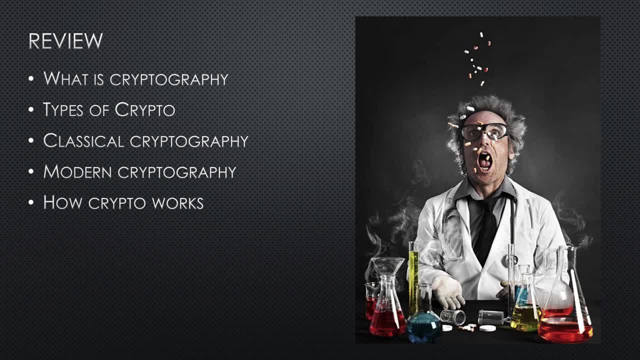 Is a very nice, gentle introduction Into what cryptography is. We talked about the two different Types of cryptography- Symmetric and asymmetric- As well as hash values. We talked about classical Cryptography. We talked about mechanical And the modern. 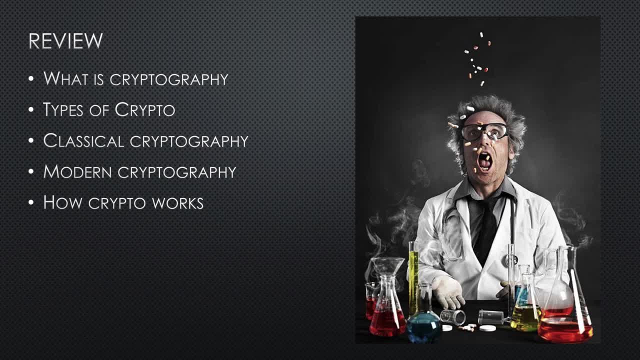 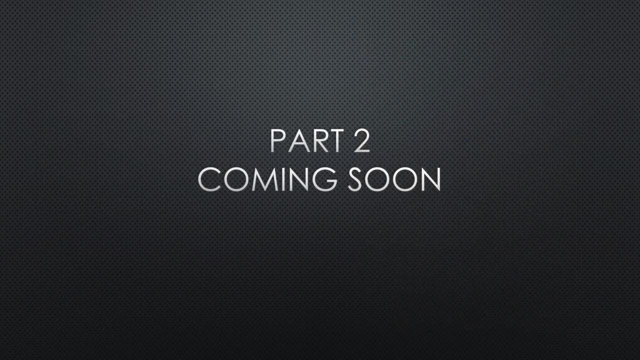 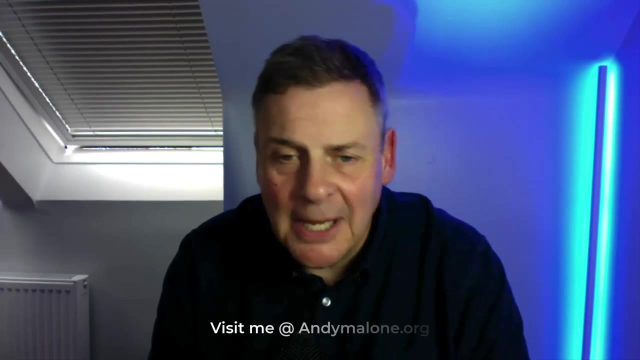 Cryptographic era And just a little bit about How cryptography works. So join me again in part two, And we're going to look at Symmetric and asymmetric Cryptography in much more detail. So there you have it. I hope you found that interesting. 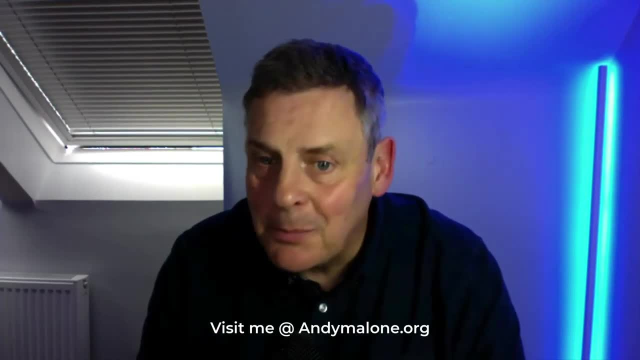 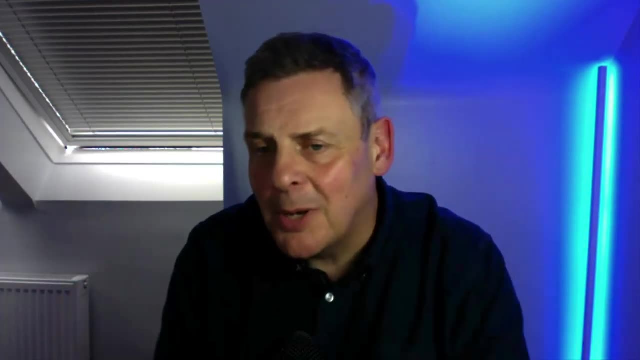 And useful And do join me again in part two And part three for this three part series. In the meantime, Any questions, any comments, Pop them down below And I definitely get back to them. okay, And as always, if you want to. 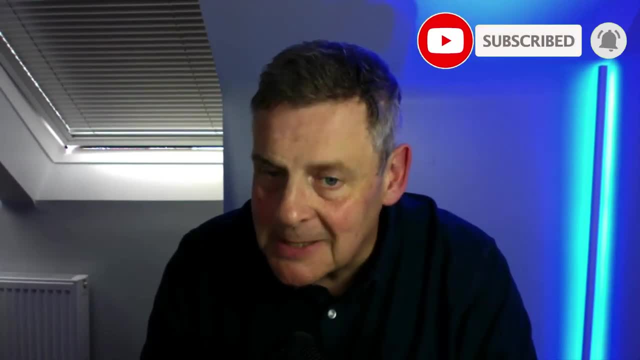 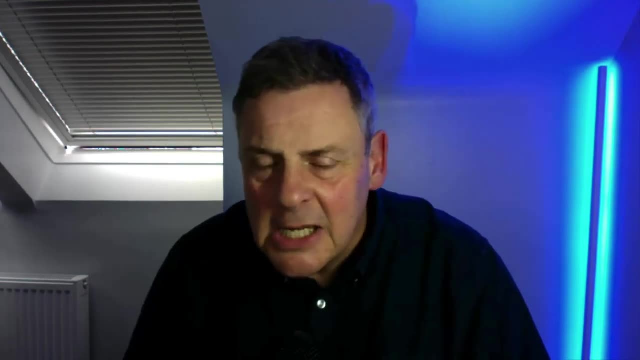 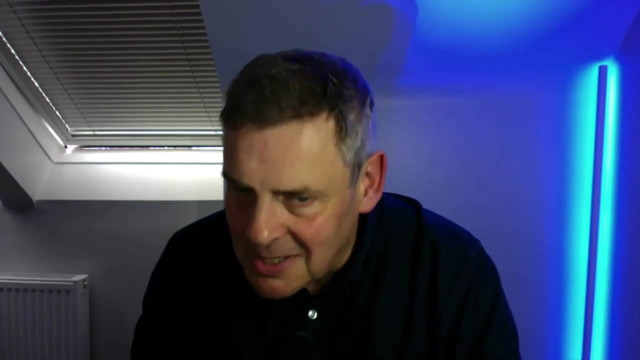 Click that subscribe button, Ring that bell And you won't miss any future postings Or any content, Any content suggestions, actually. So is there any specific topics That you'd like me to cover? I really want to hear from you. Alright, thank you very much. 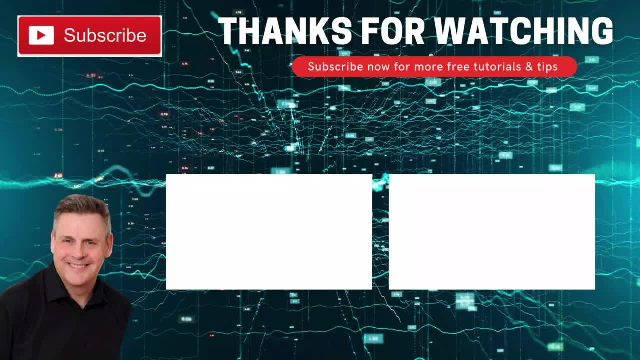 And you stay safe, And I'll see you next time, Take care. Thanks for dropping by. Hope you enjoyed the video. Go ahead and click on the subscribe button And ring that bell And you won't miss a thing. And I'll see you next time. Bye.